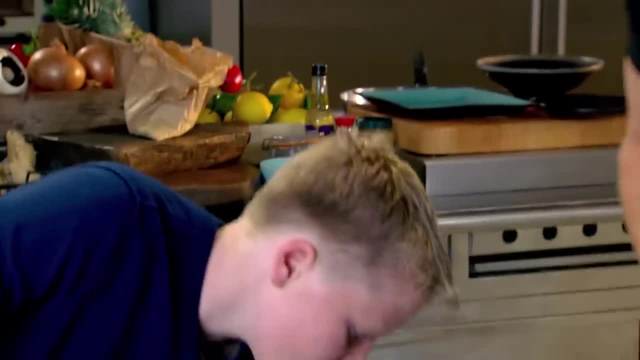 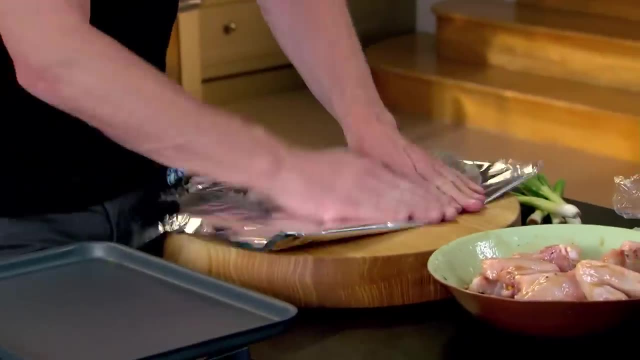 All right, so they're marinated. now, If you take the tray out, please look Bottom one, thank you, And then we're going to put some tinfoil on there, Thank you. So fold that in half. It stops them from sticking And that will stop the wings from burning. 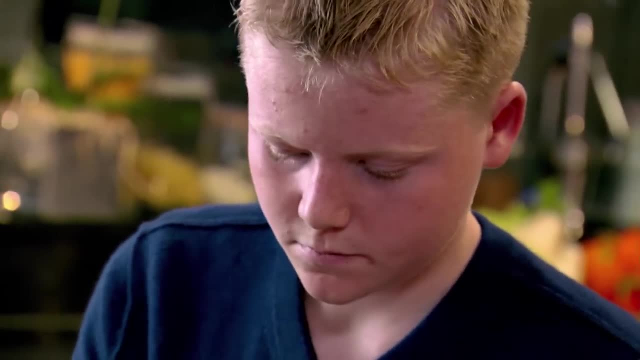 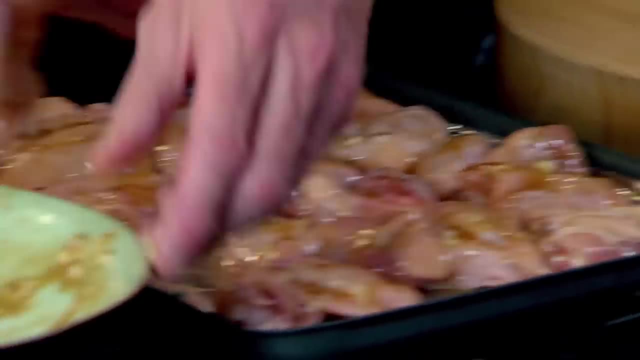 So from there, get them really dipped in that marinade And try and get the wing like that and just sort of scoop it up like that, So you get that really nice glaze on there, Mm, And then just Yeah, Mm. 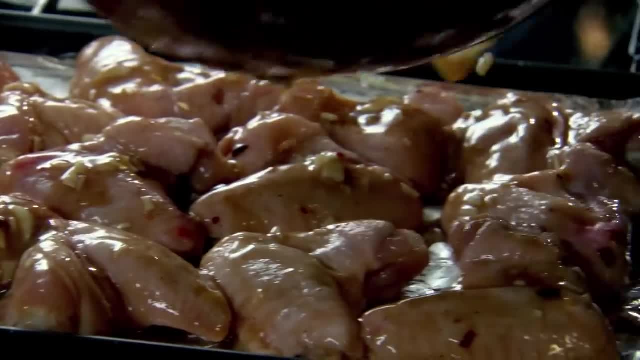 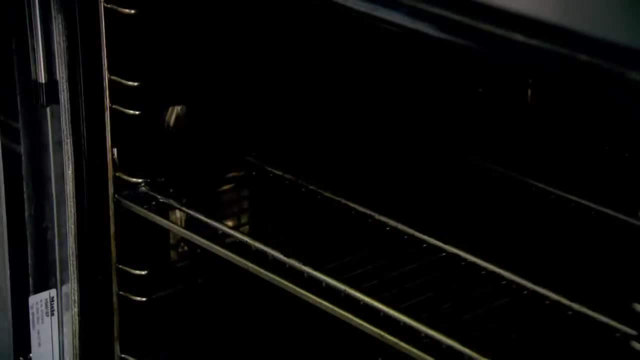 So all that garlic will roast And then we've got all those wings beautifully done. OK, mate. then ready for the oven: 170,, 25 to 30 minutes. Yep, Good man, Excellent, Nice, It's hot. 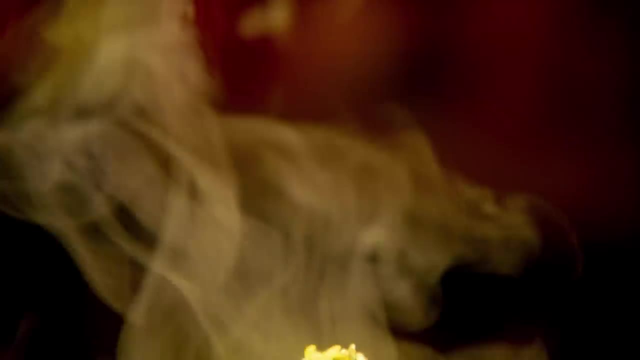 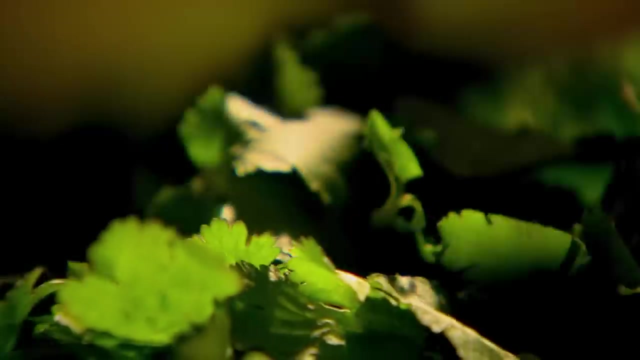 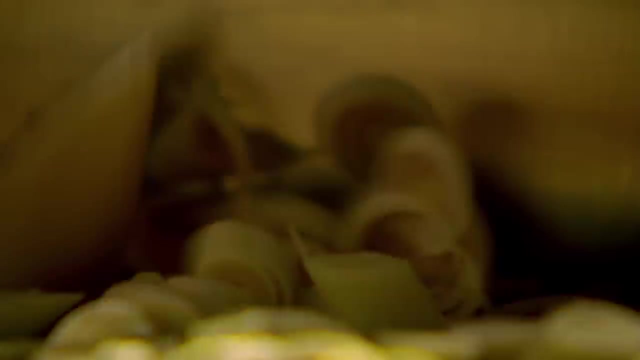 Wings are in Right To go with my ultimate Southeast Asian dinner: rice cooked in home cooking. This is homemade Thai green curry paste. For the easy green curry paste, roughly chop coriander, lemongrass, green chillies. 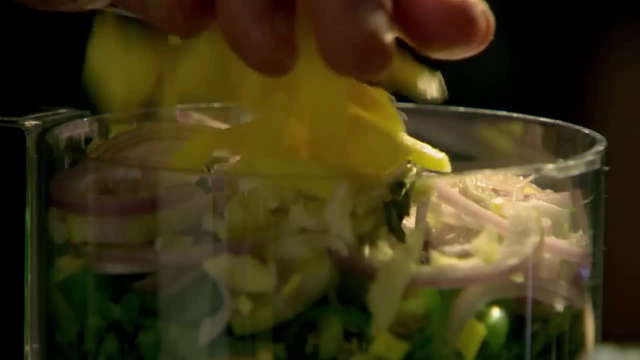 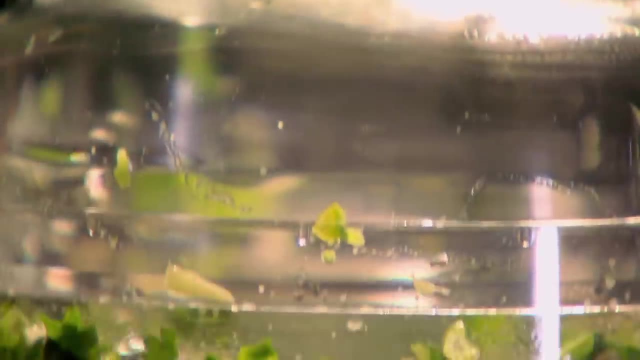 lime leaf, shallots, garlic and ginger, A glug of oil and blitz. The paste takes minutes to make, but it'll keep for up to ten days if covered with oil and stored in a sealed jar in the fridge. 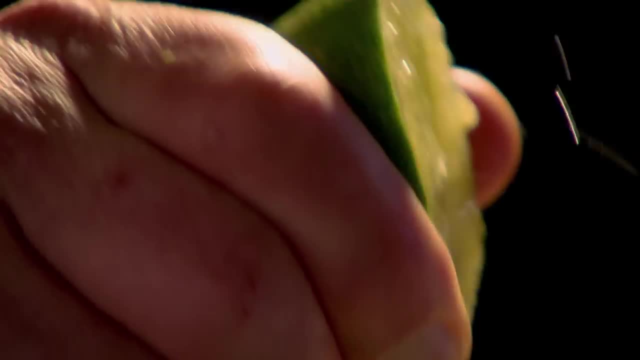 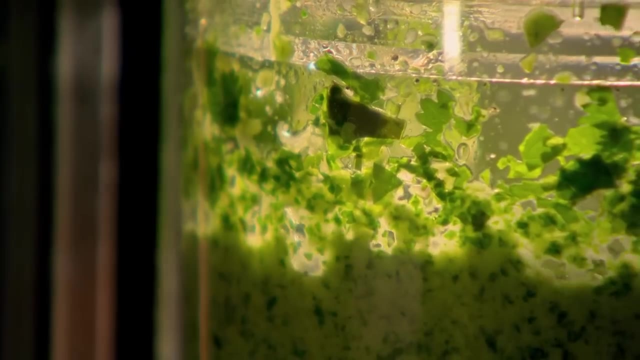 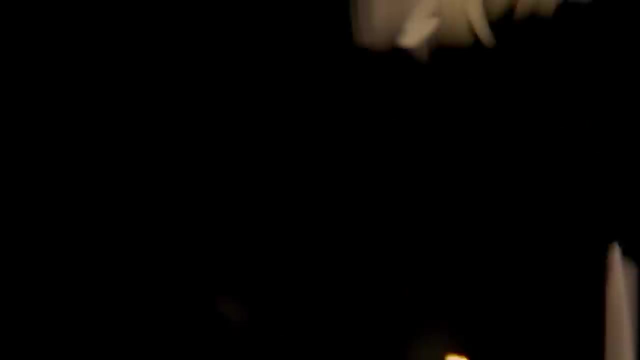 To awaken the flavours. lime roll to release the juice Next season with salt and pepper and blend into a smooth paste. Heat the paste until aromatic. Add in cooled or leftover rice. I love using fragrant jasmine rice, but your standard long-grain rice is great too. 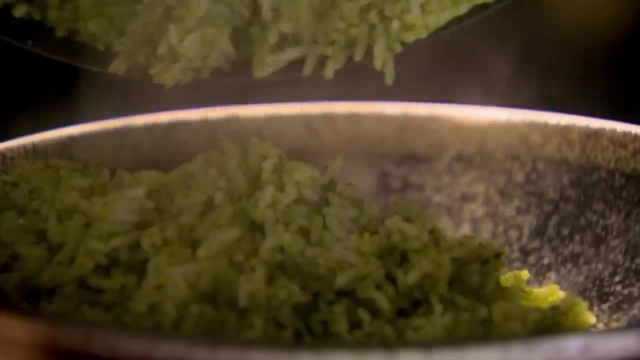 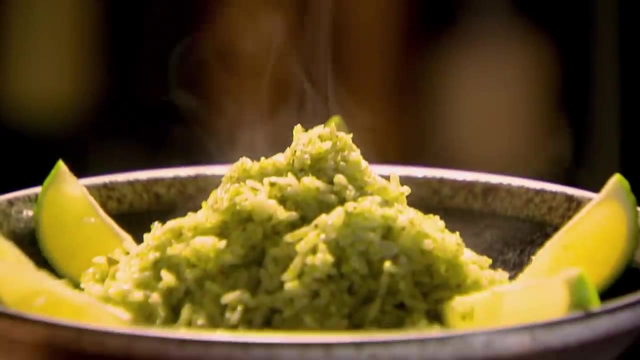 When thoroughly heated through, serve. Thai green curry paste is so easy to make, So with rice like this, it's incredible. But simply add to chicken, fish or veg to create a fantastic meal in minutes. Right now for the green beans. 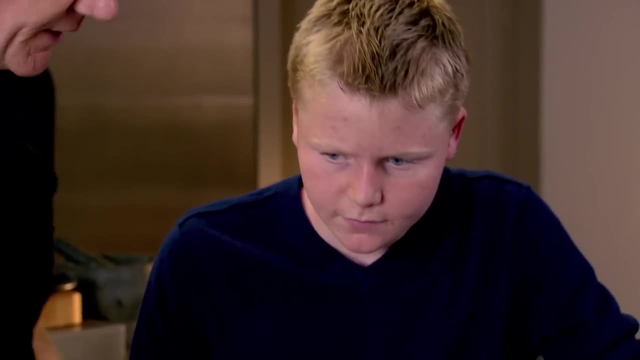 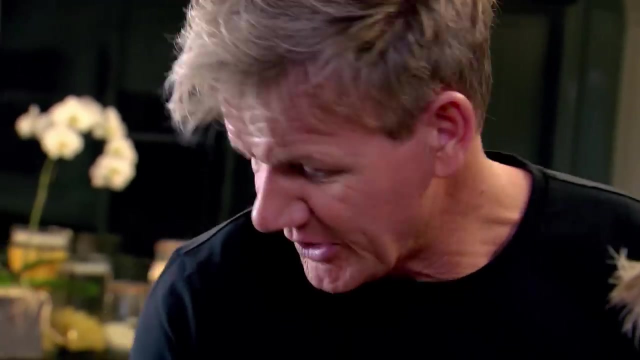 Beans in, Bring the water to the boil. What's the first thing I should put in there? Beans, Salt, Salt. So a nice pinch of salt in there, Yeah, So we'll make an amazing dressing. Two nice tablespoons, Yep. 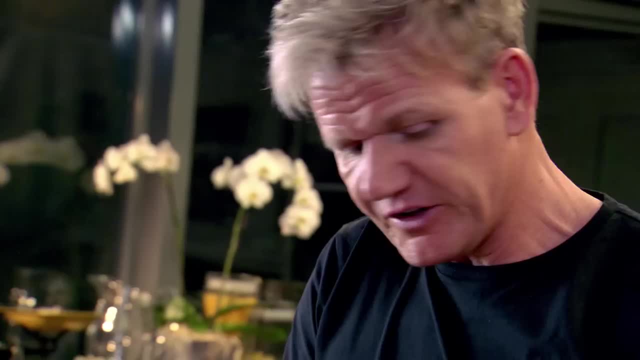 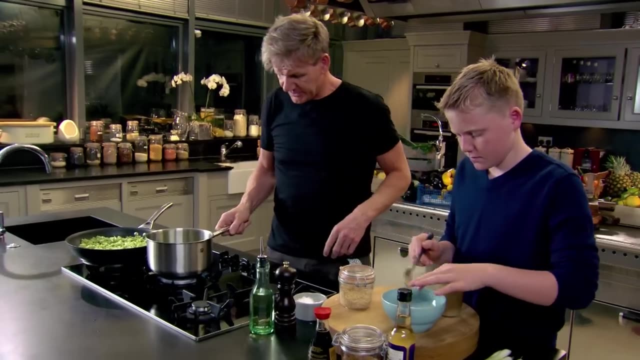 Of the crunchy peanut butter, please. Why is it crunchy? It'll give it texture and it'll be nice and sort of chunky Green beans in. OK, Got the rice, the green beans, We're going to blanch them for two, two and a half minutes. 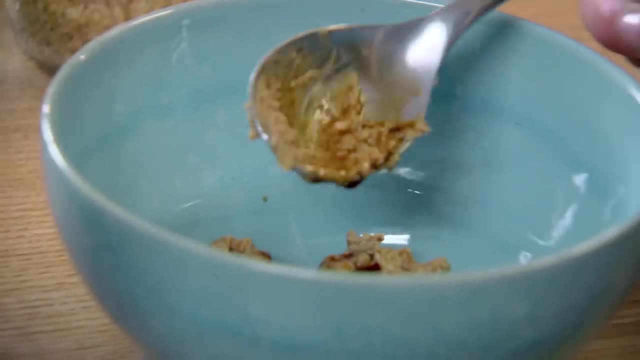 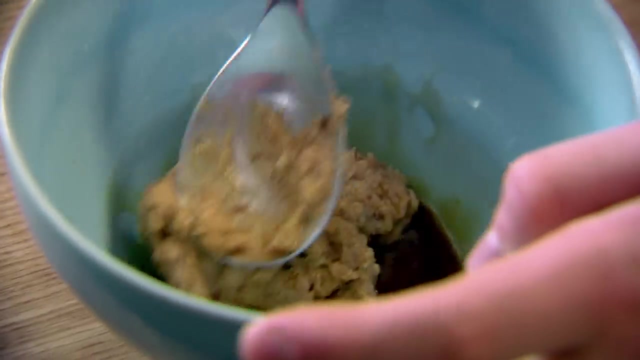 What does blanching actually mean? Blanching means, sort of part, cooking. Ah, OK, We're going to blanch them in boiling water, Yep, And then finish them in the pan. Use the back of the spoon, it'll be a little bit easier. 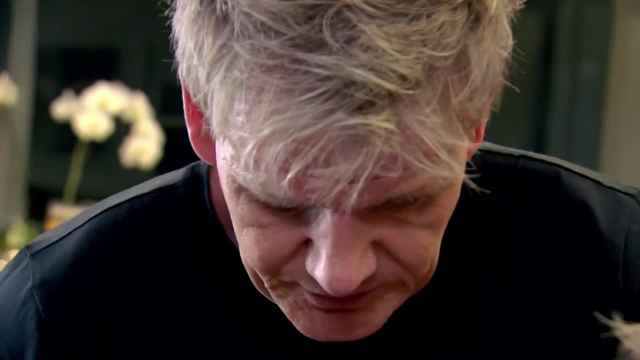 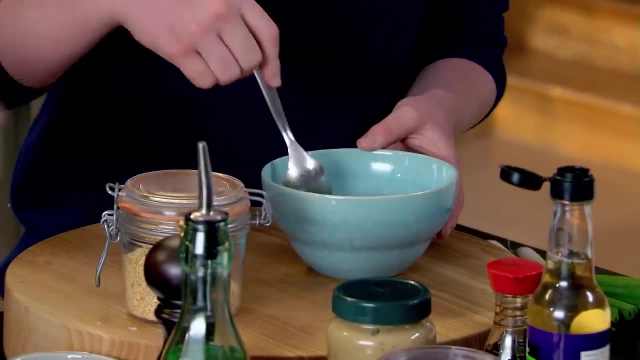 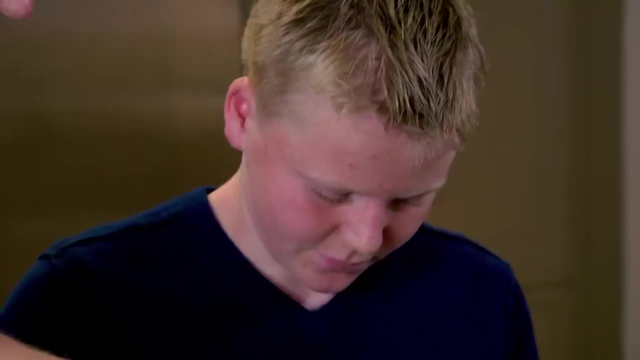 A teaspoon of brown sugar In. she goes: Nice, Is that a little bit too thick, Maybe? yeah, it is. Let's put a little touch more soy sauce in there. Let it down. Yeah, Yeah, A little touch of vinegar Nice. 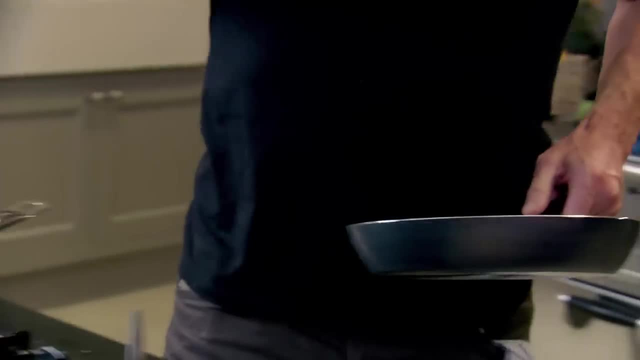 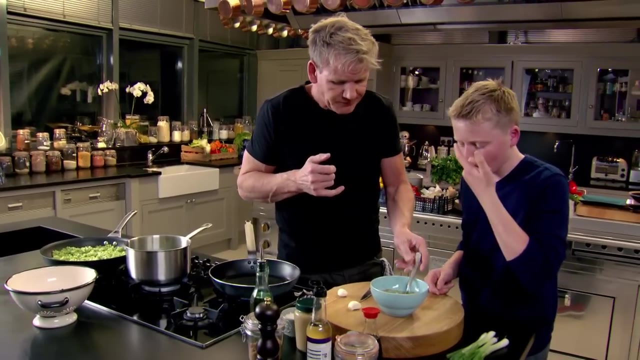 I'm going to get a pan on now for my beans. So a little taste. Can you taste it? It's so good, Oh man, Mmm, Wow, Mmm. So if you get the garlic like that, 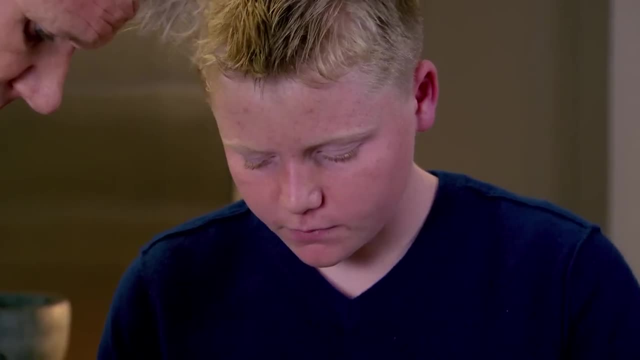 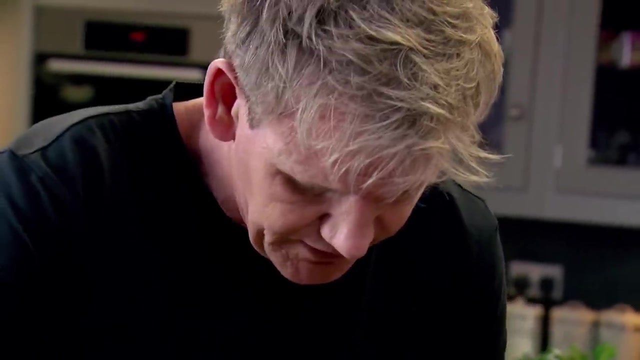 I'm going to slice the garlic down like this: Keep the knife nice and flat, That way you'll slice through it. Take your time, Don't worry about the speed. I'm taking it right first. Just cut it in half, OK. 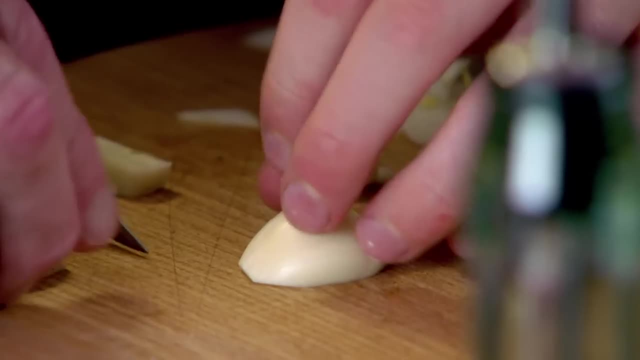 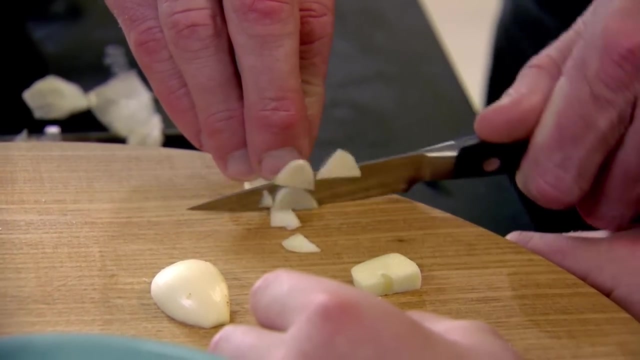 Use your fingers, Good, And then lay the flat side down, so it's nice and sturdy. And that nail there. it's not out like that, It's just guiding the knife, so you can never cut yourself like that. Good, I'll drain the beans. 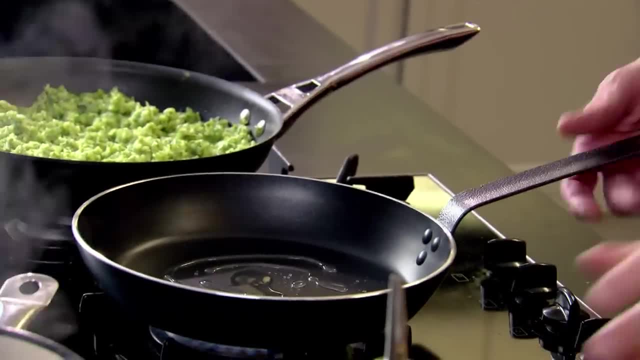 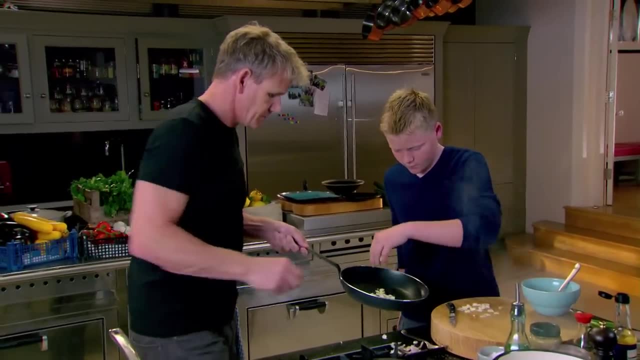 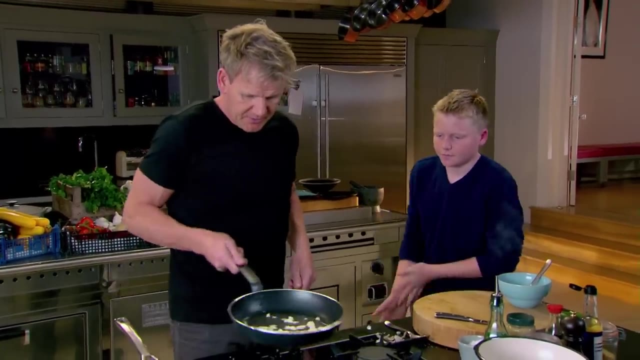 Nice, A little tablespoon I boil. Get the pan nice and hot. I'm going to throw the garlic in people. Good, Nice, Mmm. I can smell that already, Isn't it, Louis? So give that a little toss. 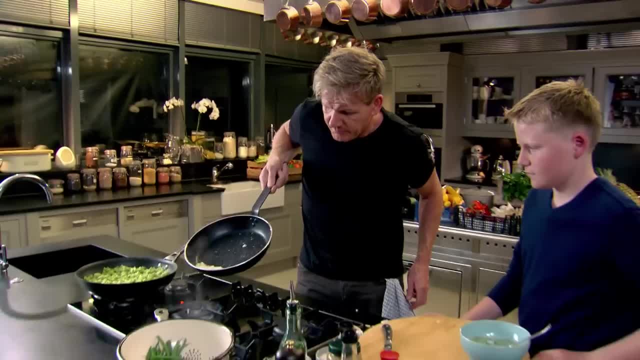 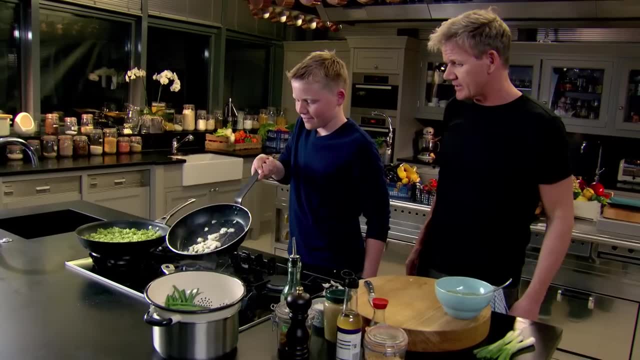 So when you toss it, push it down, push away and pull back. OK, Have a little, go Push it down, Gently, Take your time, Nice. So push down and pull back up. Yeah, That's it, Nice. 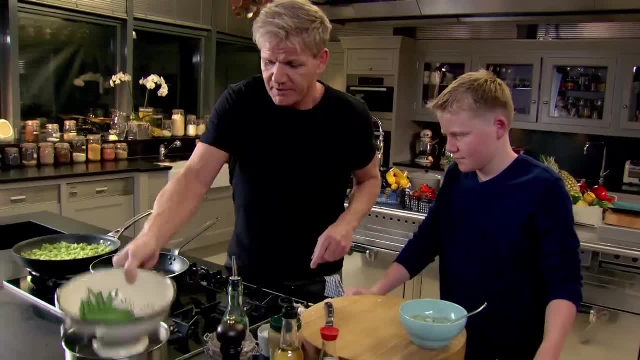 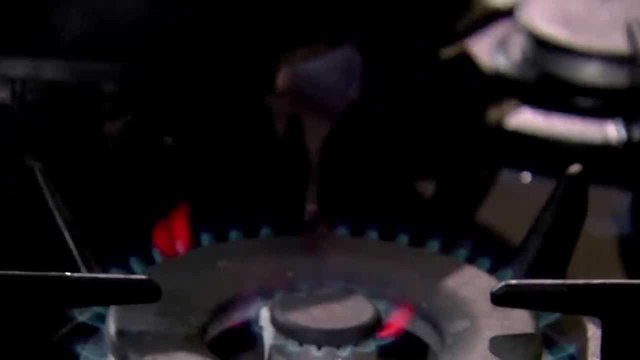 So it's getting nice and golden brown Green beans have drained and they go in. now to the garlic. Mmm, Wow, A combination of green beans, OK with the rice. Have a little smell of that, Oh, wow. 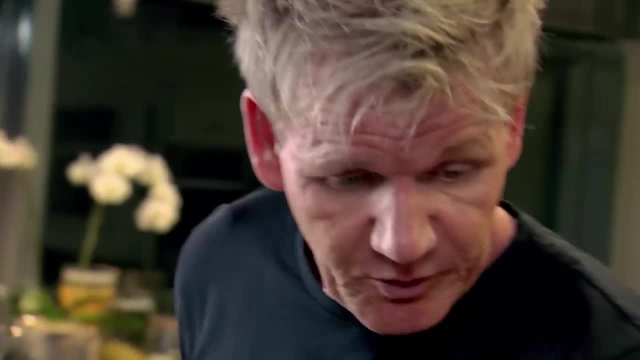 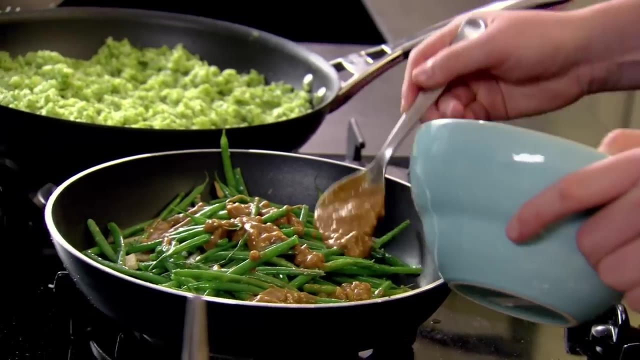 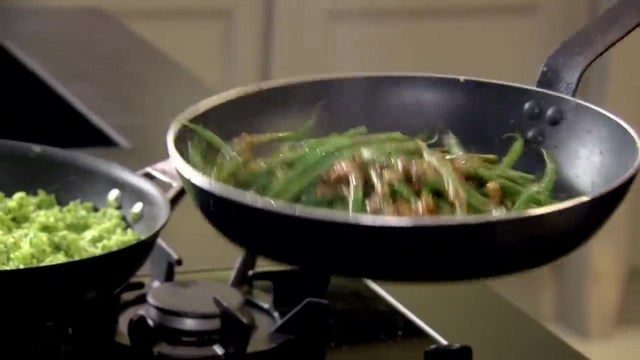 I want you now to spoon the dressing, please. In she goes. Nice, How delicious, How delicious does that look? Wow, What's Daddy's policy at home? No waste, No waste, No waste. buddy, Now Smell that now. 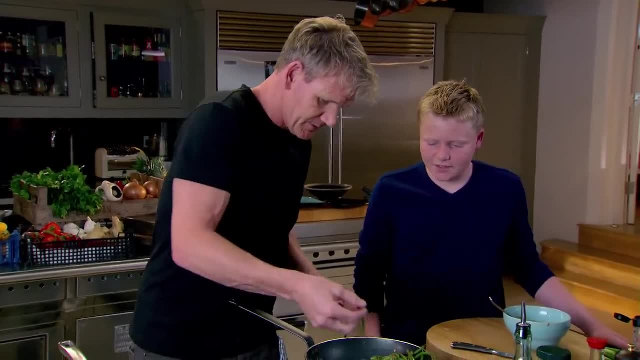 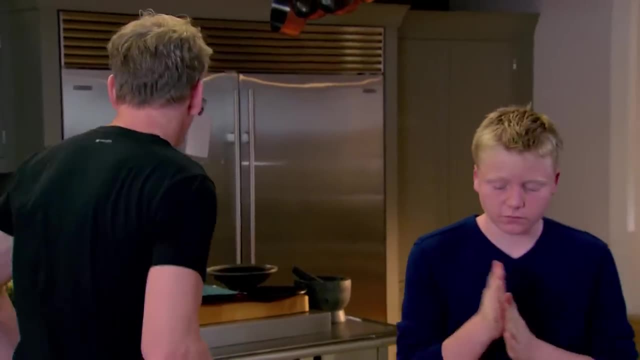 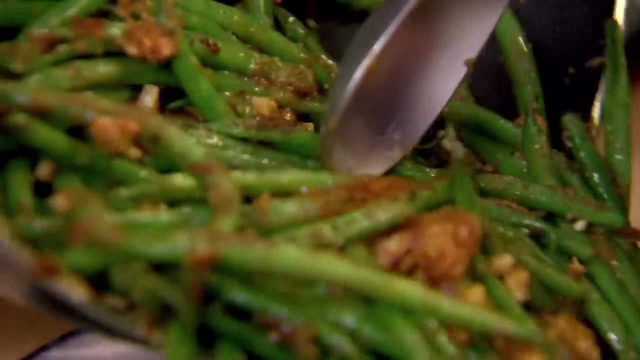 Oh, wow, It doesn't smell of green beans, it smells of No. Oh, it does. Thanks, How nice is that, Mmm? Lovely, Amazing, Right, That's the rice, that's the green beans. Now I want you to sprinkle some toasted sesame seeds on top, please. 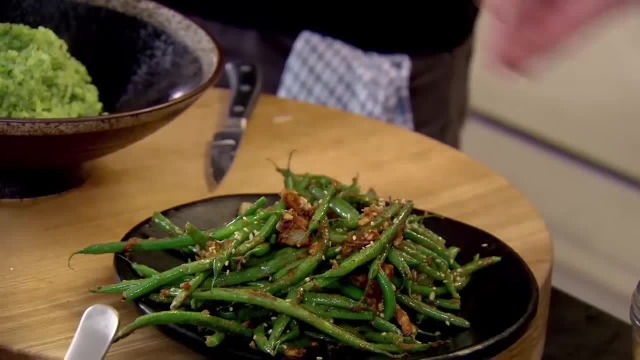 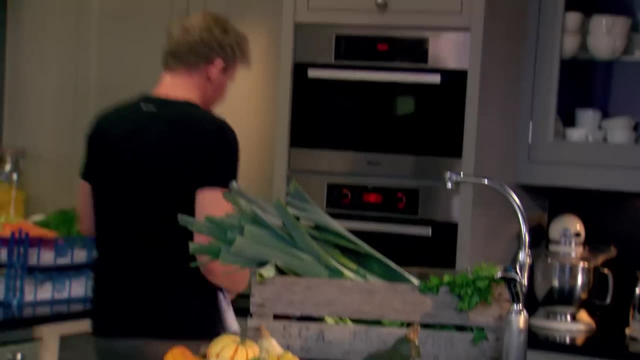 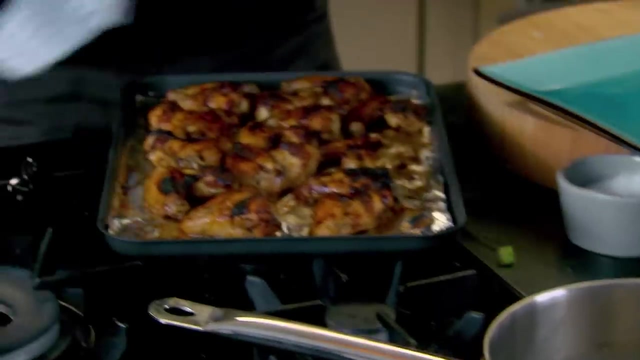 Nice and generous with the sesame seeds. That'll give the beans a little bit of a crunch. Now all that's left is for your favourites to come out. Don't those beans smell amazing? Yeah, Mmm, Mmm Jack, look at those beauties. 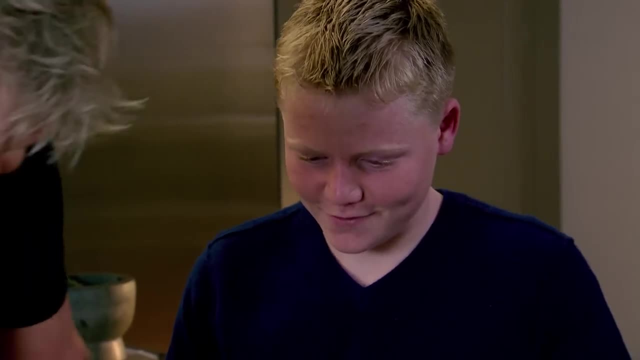 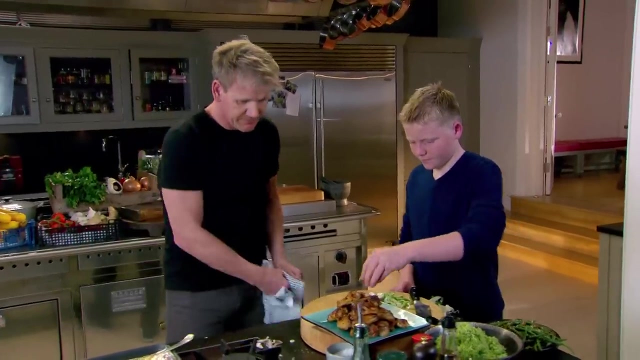 One for me, one for you, Three for me, one for you, One for you. Now I'd like you to sprinkle some spring onions Cool on top, please. Nice and generous, You've transformed a very cheap and cheerful chicken wing. 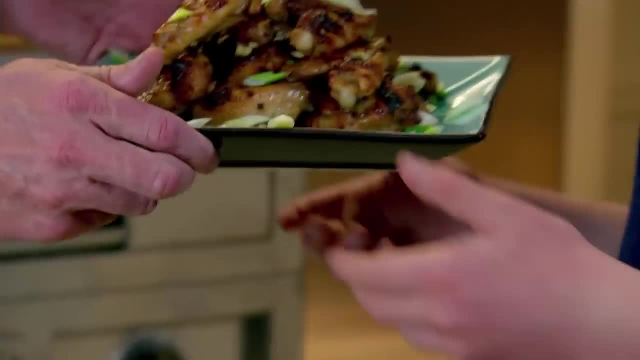 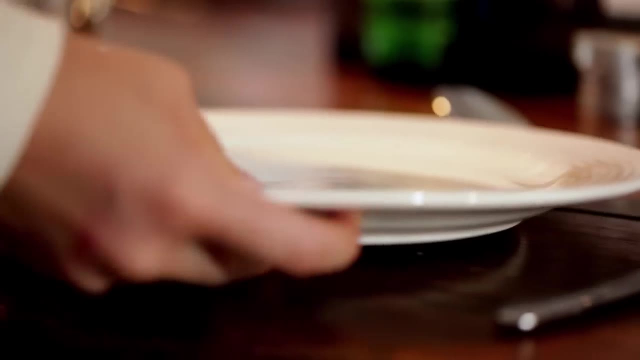 Yeah Right, I'm going to take them over. Please do not drop them. OK, Jack, That's good bud Nice. This is my ultimate simple South-East Asian dinner: Sticky spicy chicken wings, Thai green curry rice. 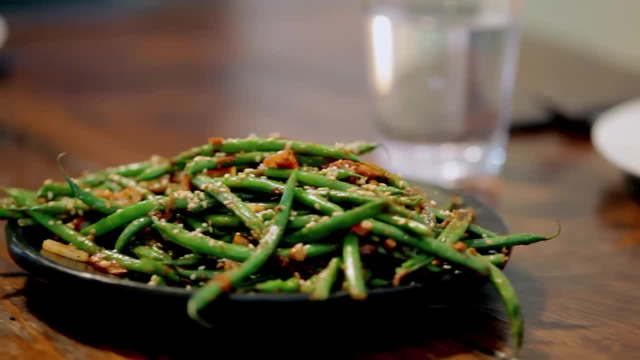 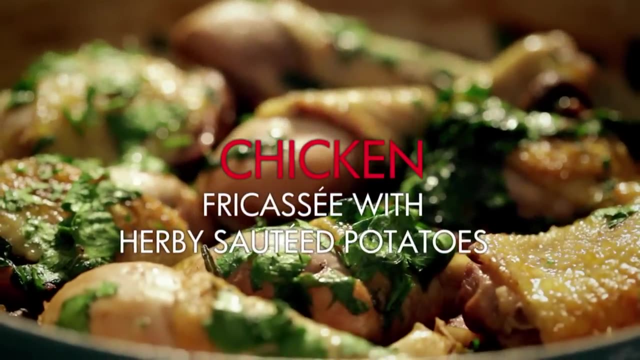 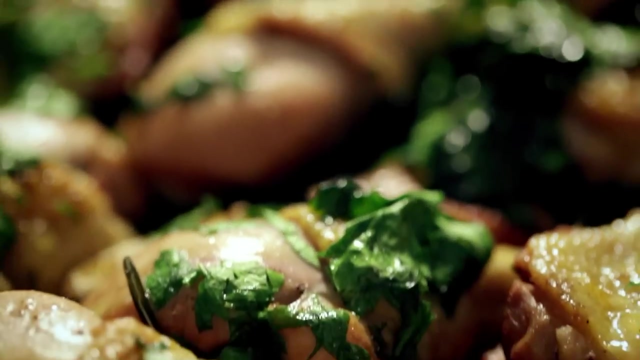 and fantastic beans with chicken Chilli peanut dressing. guaranteed to get the fussiest of eaters into greens. Made with fantastic chicken cooked using a classic but simple French technique. this is my ultimate home-cooked French dinner. First job: my chicken fricassee. 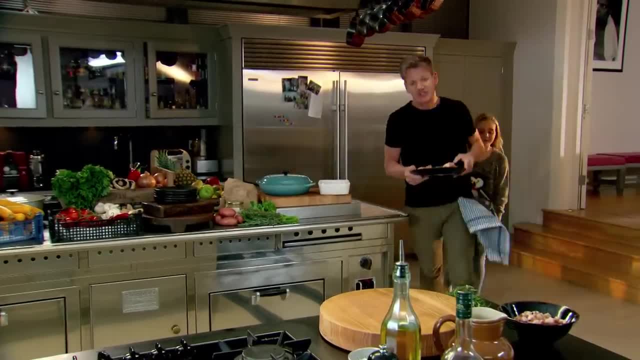 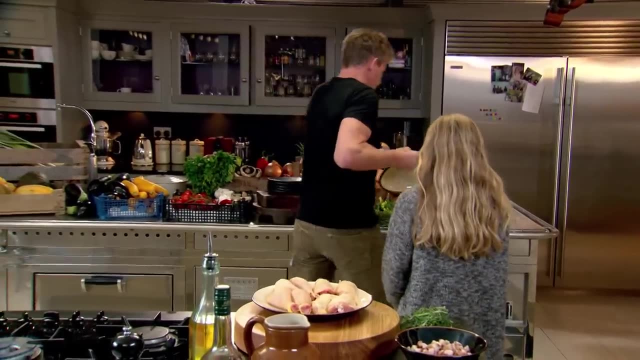 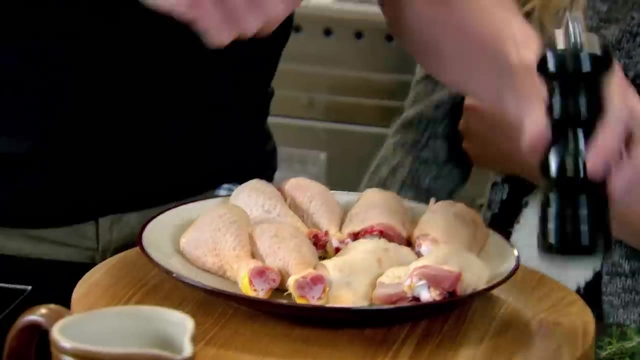 Tilly, would you mind helping Daddy with the chicken fricassee please. We're going to start off with browning all the chicken off nicely, Pan on, Get that nice and hot. What I want you to do for me first is to season the chicken with salt and pepper, please. 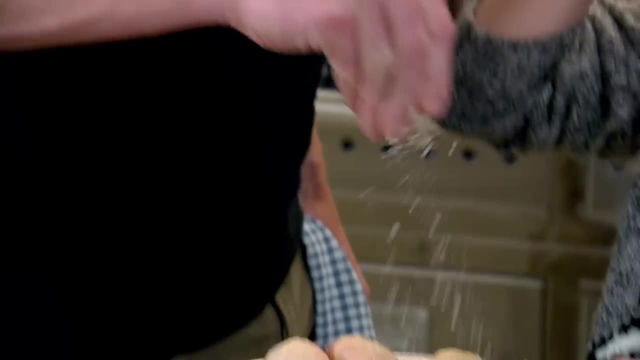 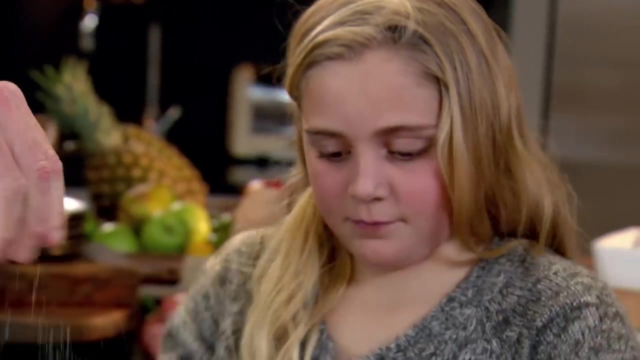 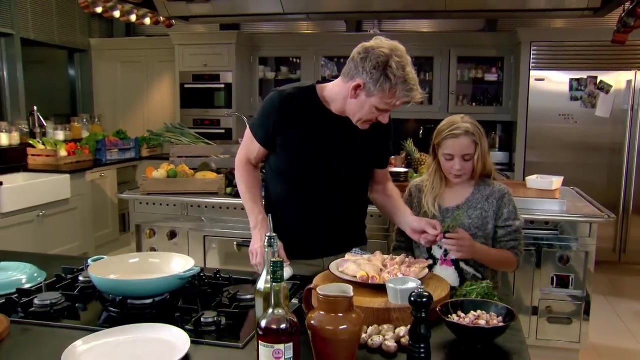 Thank you. So that's on one side. Then we turn the chicken over, So we season it on the other side: Salt, Good girl, And pepper- Nice. Now this is almost like a chicken stew. OK, What's that there? 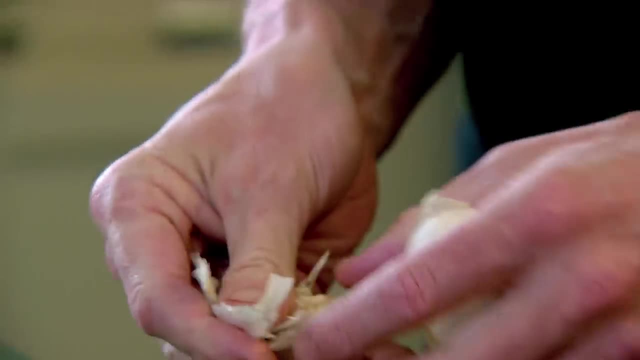 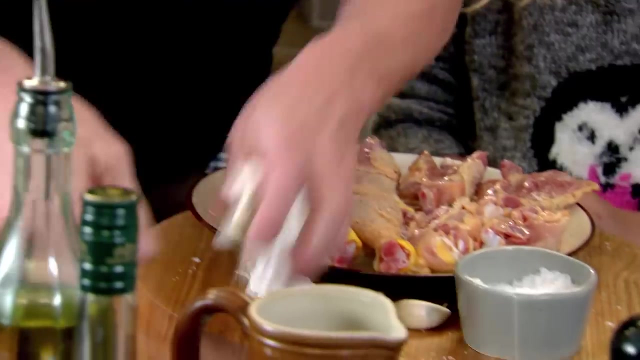 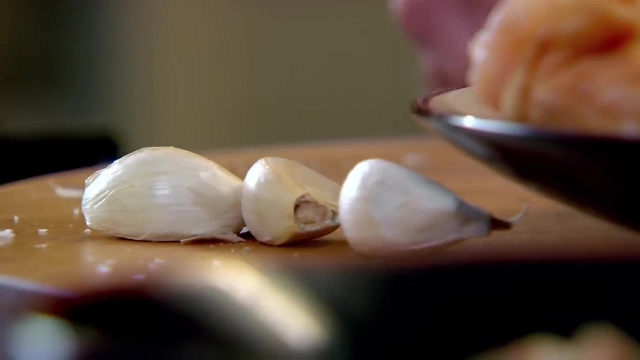 Mmm. thyme, Thyme, Good girl, What's that one there? That one's rosemary. That's right, rosemary. And because this is quite a rustic French dish, we don't need to chop everything, So you get the garlic. 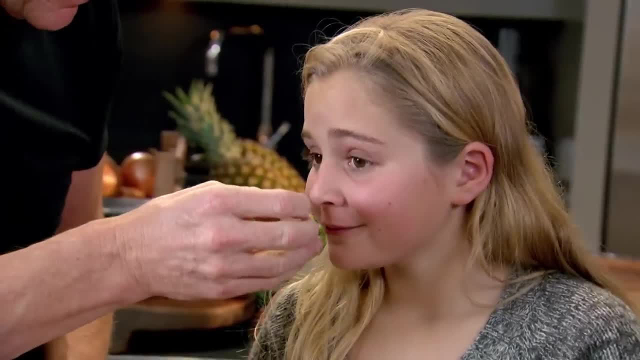 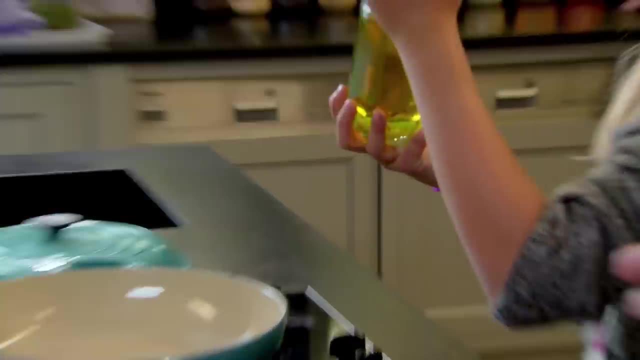 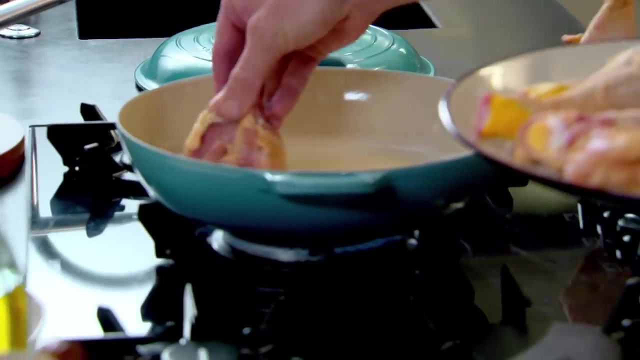 and you just bash it like that. Now smell Mmm Right. So that's nice and hot. Put a tablespoon of olive oil in there, Couple of glugs, One, two, Good girl, Put the chicken in And you lay away. 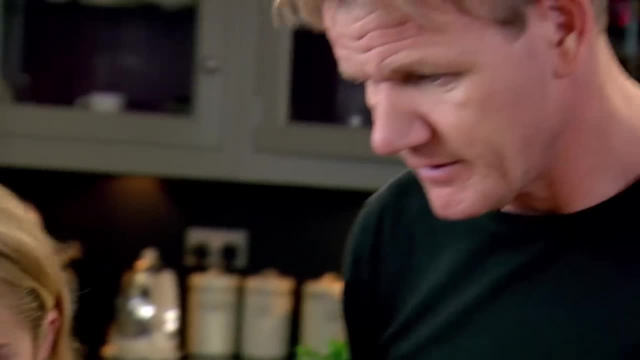 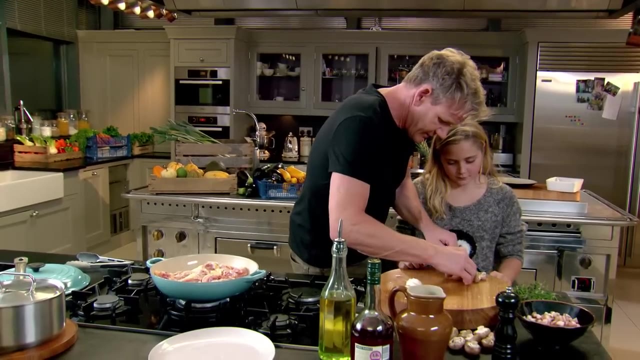 You get that nice and brown. You're getting good at this. You are Skin side down, So we get the colour on the skin. Now I just want you to cut the mushrooms in half for Daddy, please. Thank you, These are chestnut mushrooms. 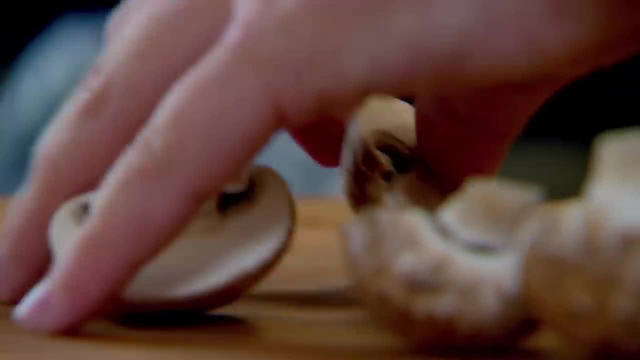 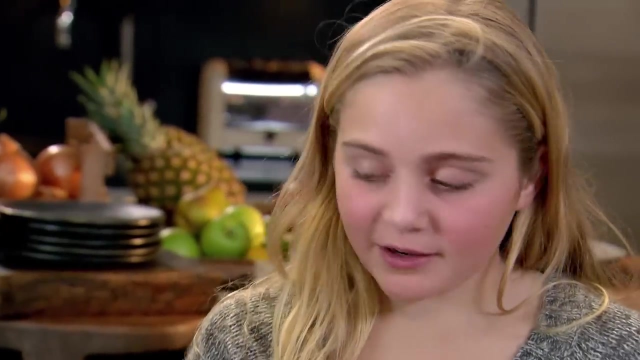 There are lots of different types of mushrooms, aren't there? There are lots and lots of different types of mushrooms. Which one's your favourite? One of my favourites is the Giraud mushroom. I like mushrooms that are a bit bigger than this. 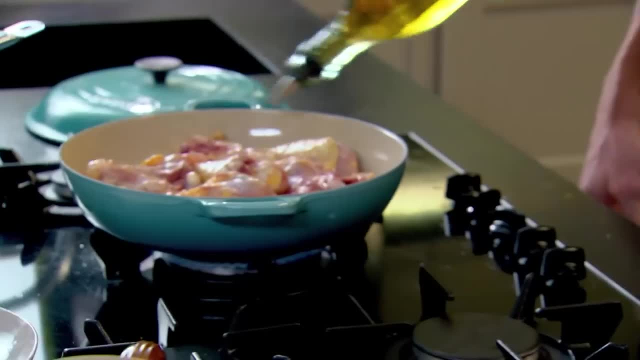 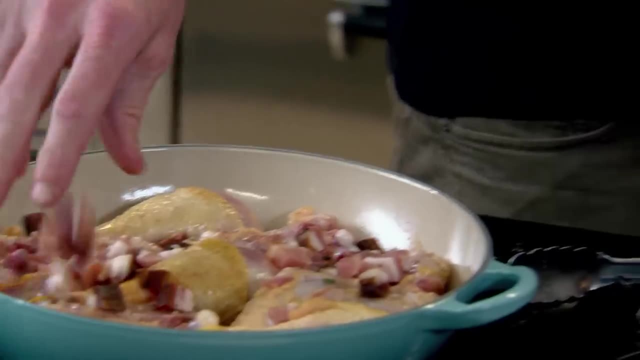 And some dinners with Mum. we cut out the middle, put pesto and cheese in it, and then we bake them. Oh, So I want you to sprinkle the pancetta over the chicken, please, Good girl, Nice, Have you got the mushrooms in? 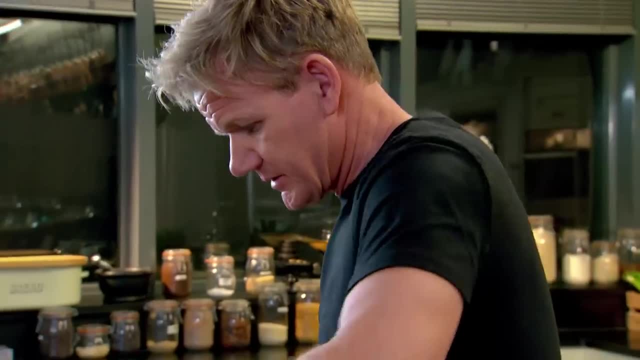 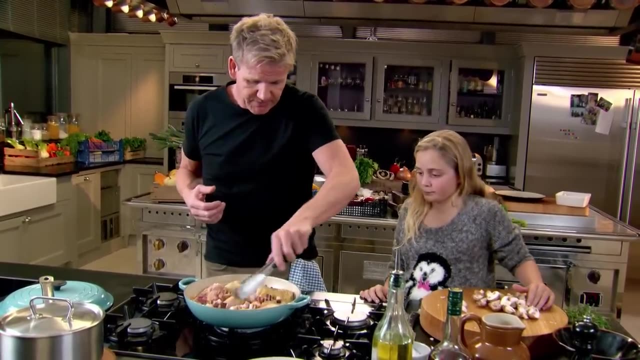 Not yet, because I'm going to get some colour on the chicken first. OK, And as that pancetta starts to cook down, it puts a really nice flavour On the chicken. Yeah, So we're sort of sautéing everything, OK. 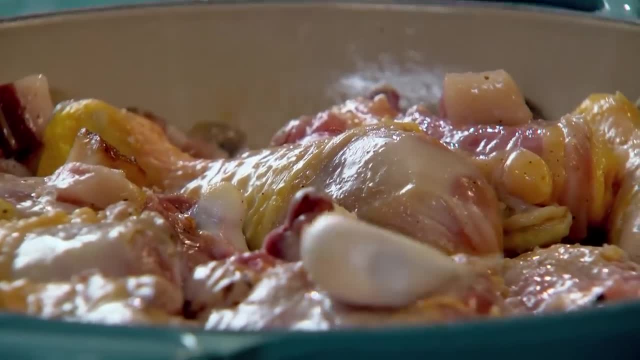 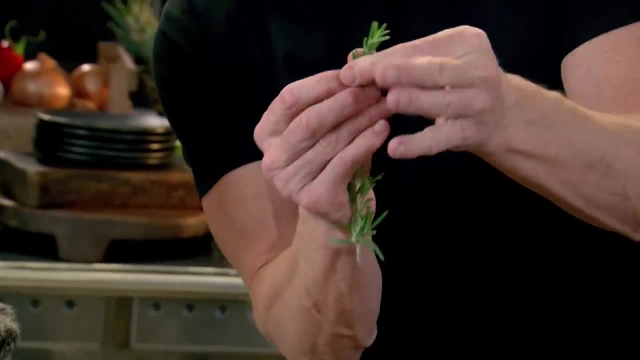 Right, garlic in. please, Good girl, Just throw them in Now. I want you to sprinkle the mushrooms on top of that, Good girl. And there's the rosemary. OK, you get your fingers like that and you pull it down. 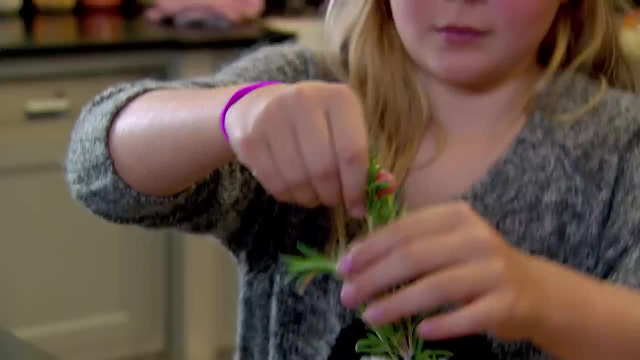 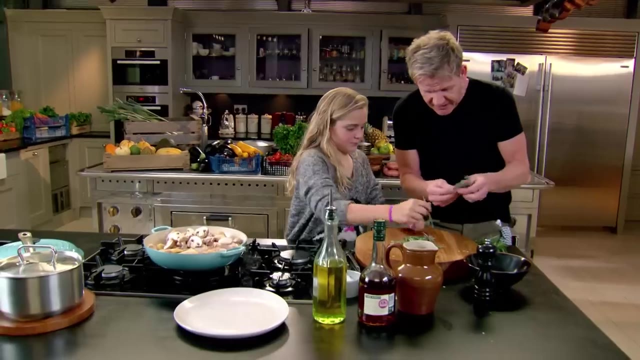 You take it all off, Hold it, Put it down, Good girl. So now you've got the nice little rosemary sprigs, And we do the same with the thyme. Now the thyme flower's a little bit smaller. 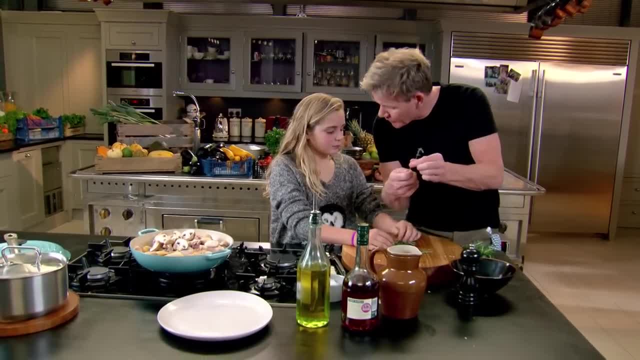 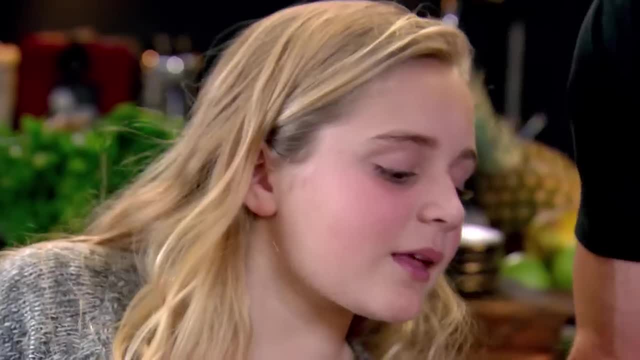 What different flavours do they give? So the thyme is a little bit sweeter, OK, And the rosemary a little bit more savoury. Which ones do you like? I like them both because they both give a nice flavour. 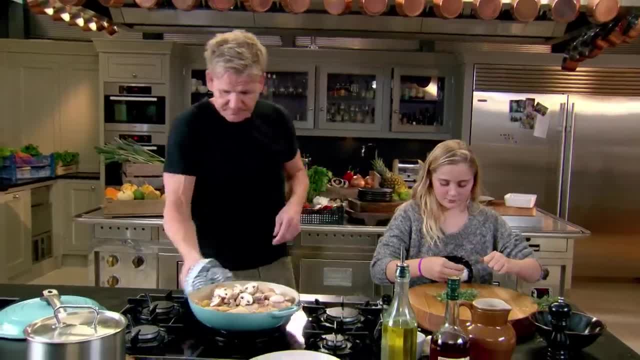 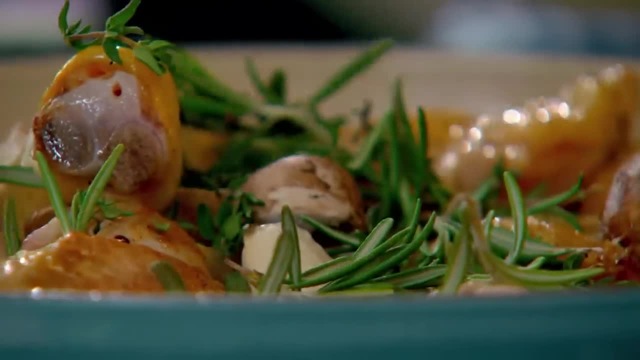 Don't they? So bay leaf in. I'd like you to put that rosemary and thyme in there. please Lovely Sprinkle it over, Right? I'd like you to stand back now, because we're going to flambe this. 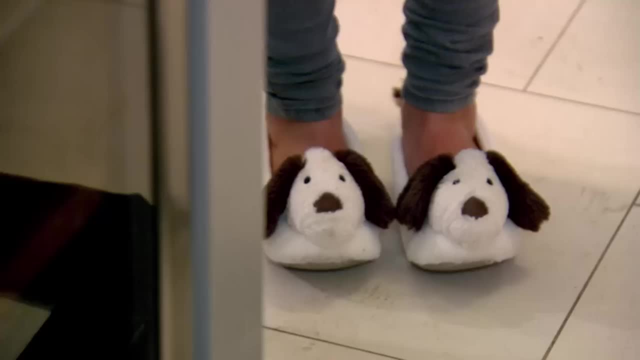 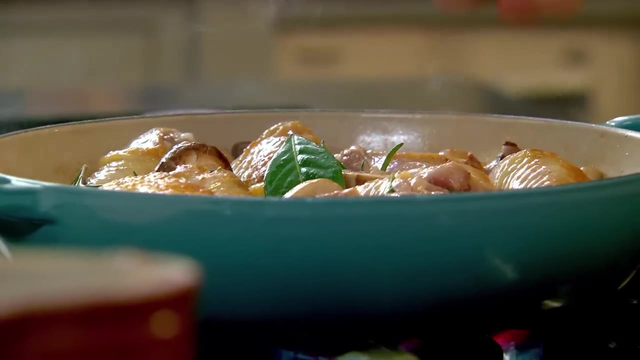 I do not want to get those little slippers caught on fire. What are the names? Rumpel and Judith, Judith, Nice, OK, great, Ready, Yeah, In with the brandy And then just tilt the pan gently. 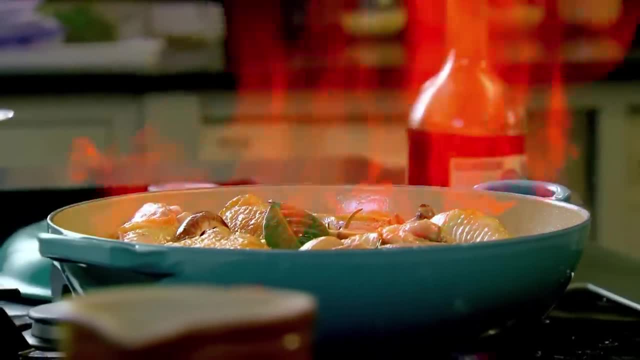 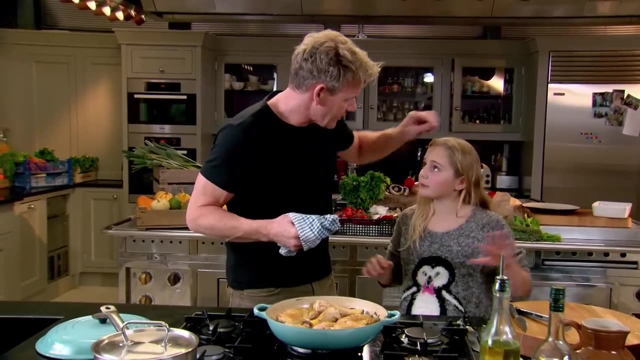 Whoa, Whoa. How cool is that, Isn't it? magical, Beautiful, A bit like a cauldron. All the cognac has been flambeed, So there's no raw alcohol anywhere, So we've got a really nice, deep, rich flavour. 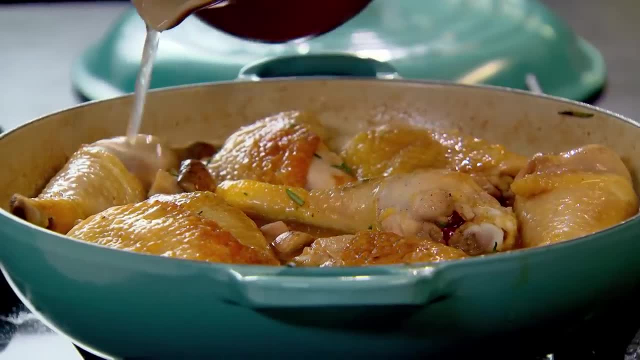 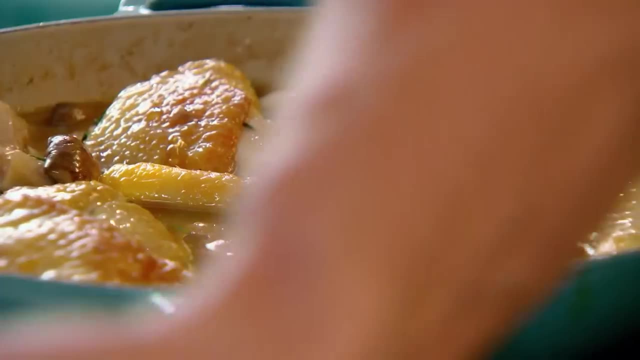 I'm going to add my chicken stock. You know, Rumpel likes that, Not my slipper, Rumpel. Rumpel the dog. Ah, Rumpel the dog, Well, he likes chicken stock. Yes, When he's a good boy, he gets it with his biscuit. 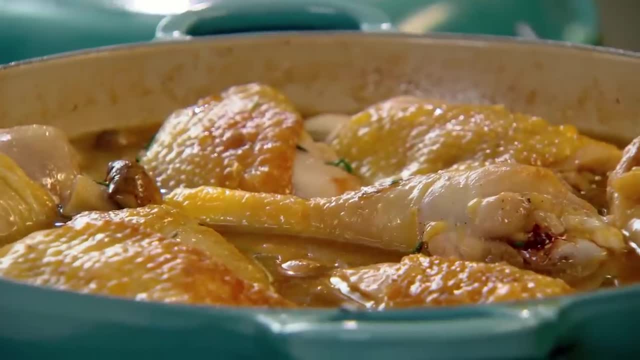 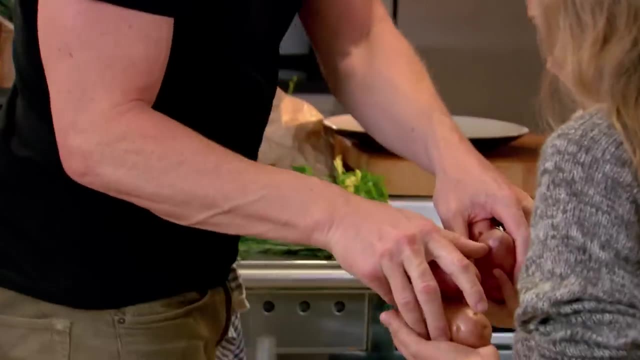 It's gone in like wow, really quickly. Simmer and reduce the stock for around ten minutes. Now we're going to cook the most amazing potatoes. Sautéed potatoes are really simple to make and absolutely delicious. Start by slicing the potatoes into finger-width pieces. 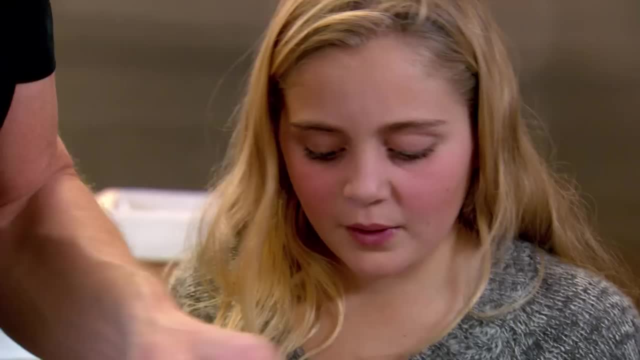 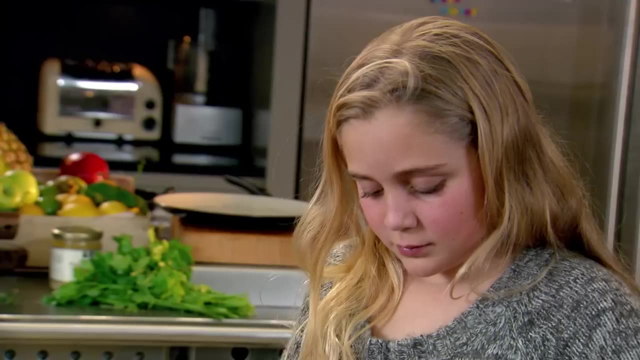 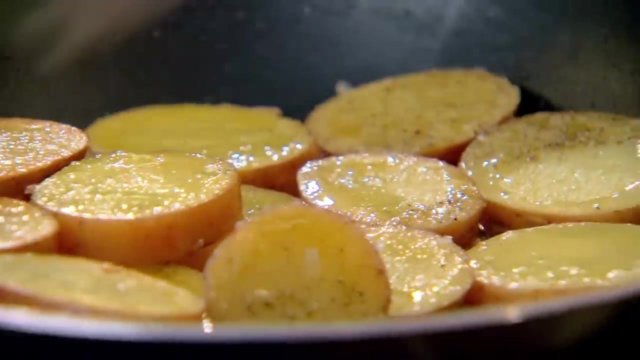 Then parboil them for five to six minutes. When you cook something like rosemary or thyme or basil, does it slowly let off the flavour into the hot oil. Very much so. In a hot pan add a tablespoon of goose fat and sauté the potatoes until they turn golden. 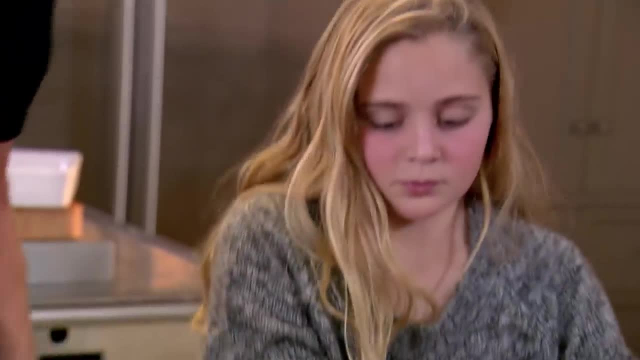 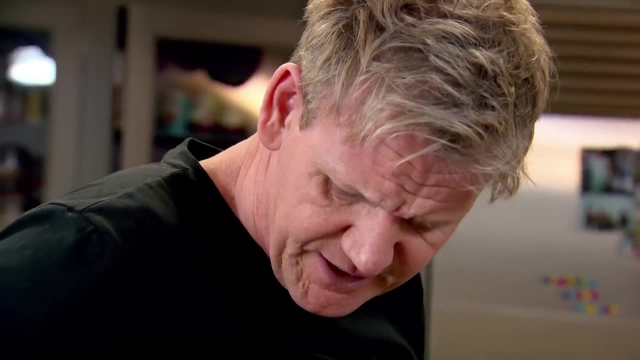 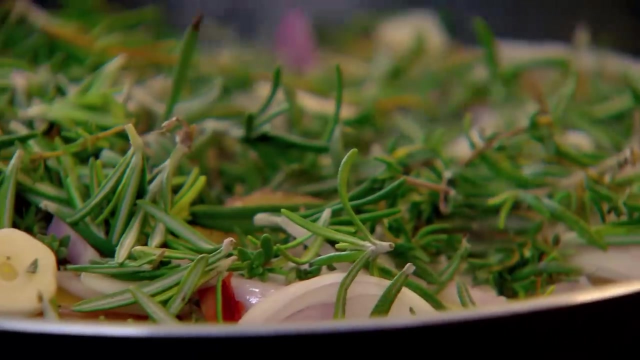 And add in shallots, garlic, rosemary and thyme. That goes in over the top And that goose fat now is starting to fry the potatoes. You just leave that sat there To complete my ultimate French dinner, my version of a classic. 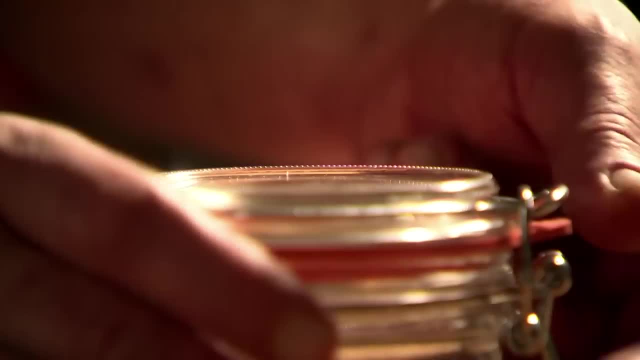 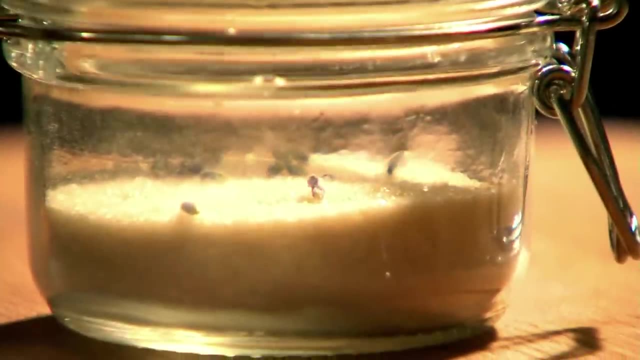 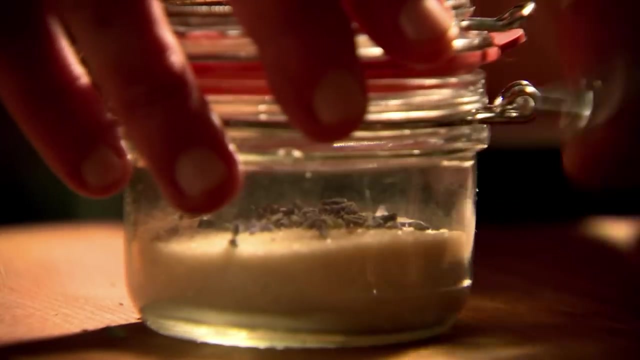 A glorious lavender creme caramel for dessert. The first job is the lavender sugar. You can buy this ready-made or simply add dried edible sprigs of lavender to caster sugar and store. You can also try this trick with vanilla pods and cinnamon to bring new subtle flavours to sweets and baking. 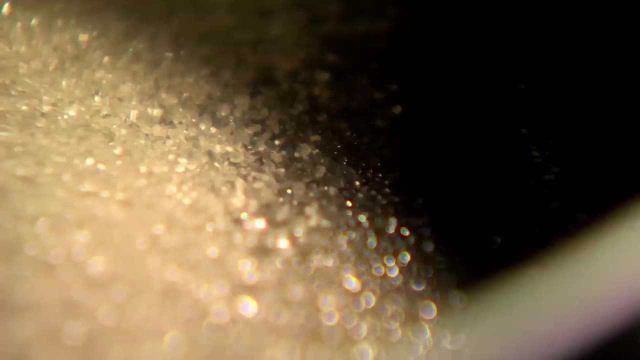 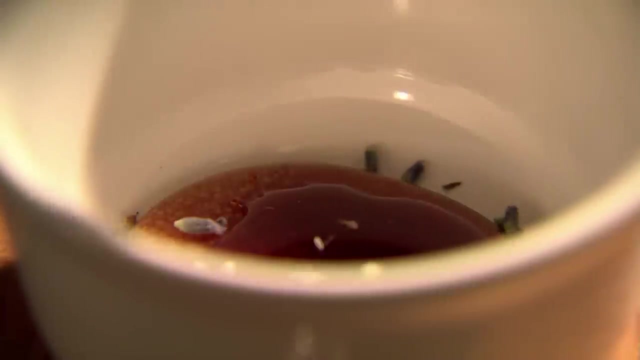 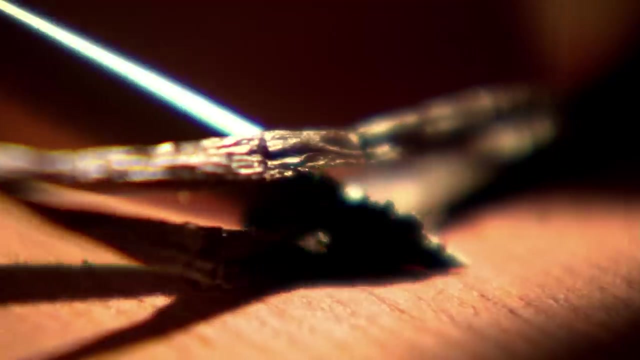 For the creme caramel. melt plain caster sugar until it turns dark golden. Pour into ramekins, sprinkle with lavender flowers and cool. Now to make a simple custard: gently heat whole milk in a pan until steaming. Meanwhile whisk together egg, vanilla seeds and lavender sugar until golden and fluffy. 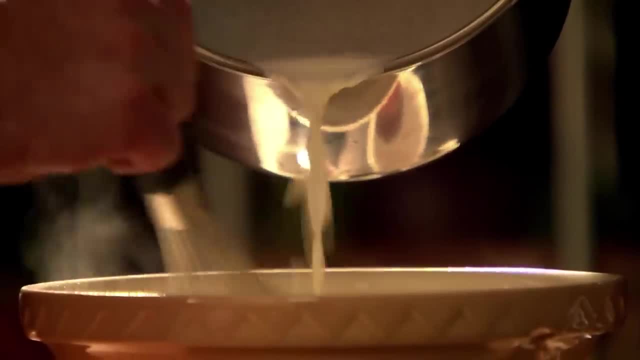 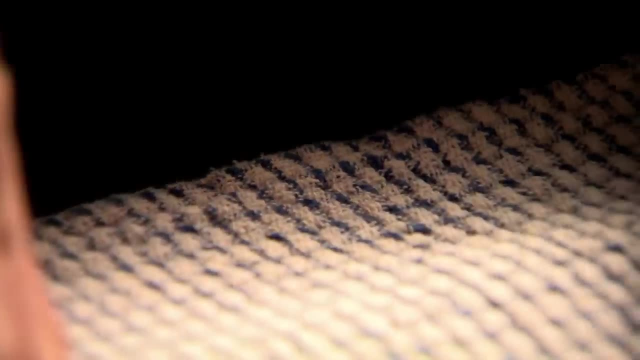 Then gradually pour the hot milk into the mix, whisking continuously until the custard is smooth and creamy To set cook in a water bath or bain-marie. A good tip is to line a roasting tin with a cloth to stop the ramekins jiggling around. 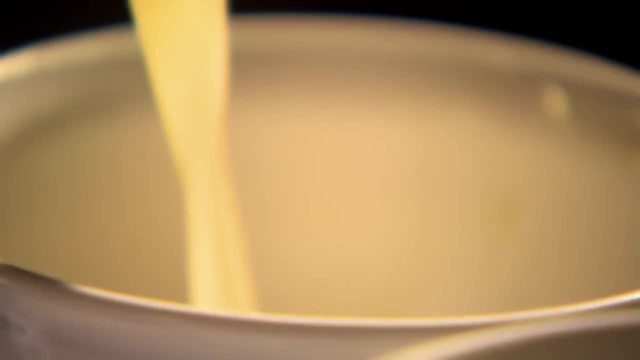 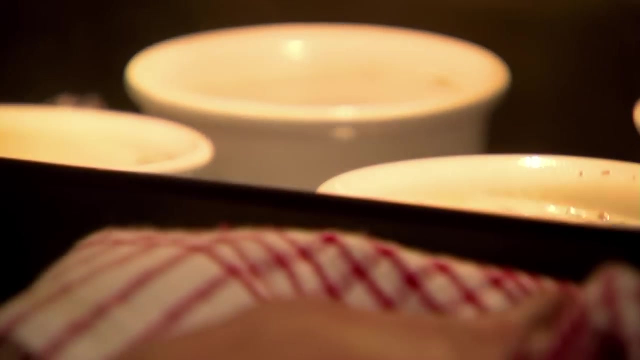 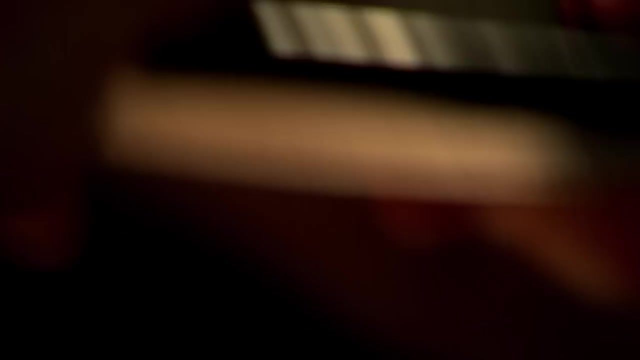 Pour your custard, then boiling water around the ramekins until halfway up the sides. Then cook in a preheated oven for around 30 minutes until set Cool in the fridge. then, when you're ready to serve, dip the ramekins in hot water to loosen the creme caramel. 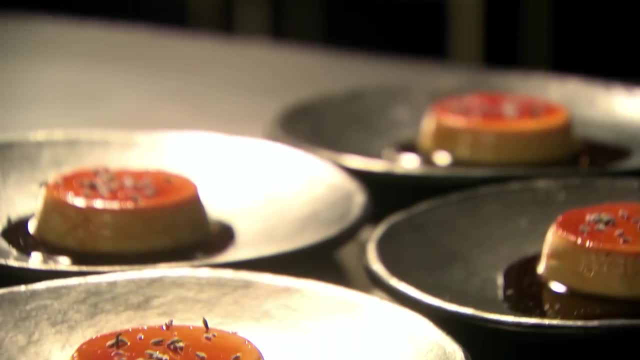 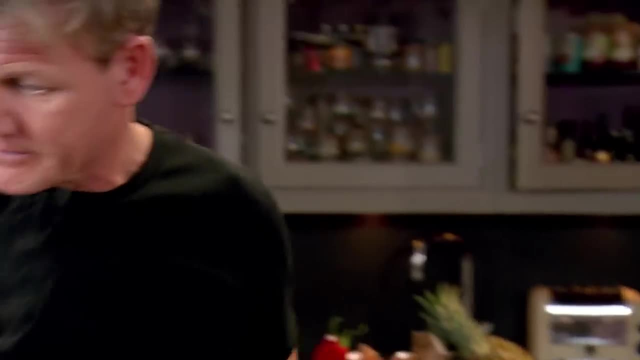 Et voila, Lavender creme caramel. Look at that chicken now. So I'm just going to turn the gas right down and put the lid on, Just like that, but leave a little bit So it can let out some steam. 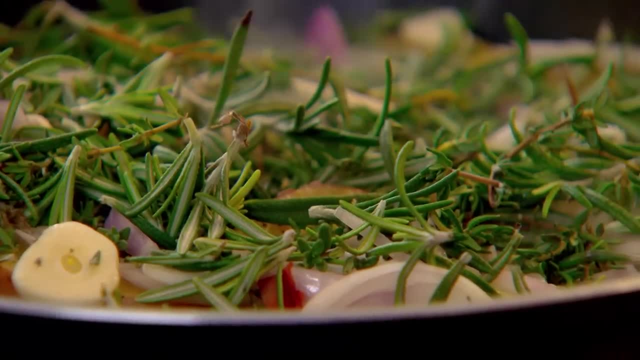 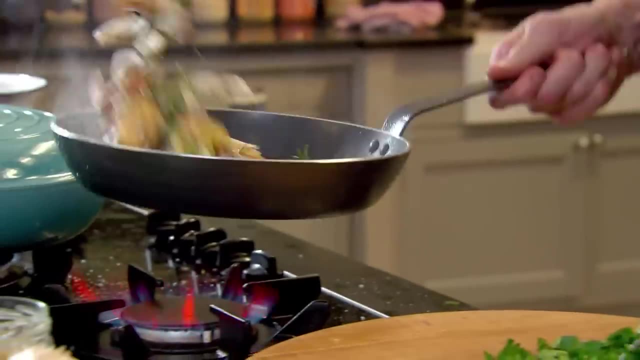 So it can let out some steam. that's right Now. what I'd like you to do is to chop, Deli some parsley, Crunch it up nicely, tuck your fingers in and take your time. Mmm, It turns, you've got lots of different flavours in there. 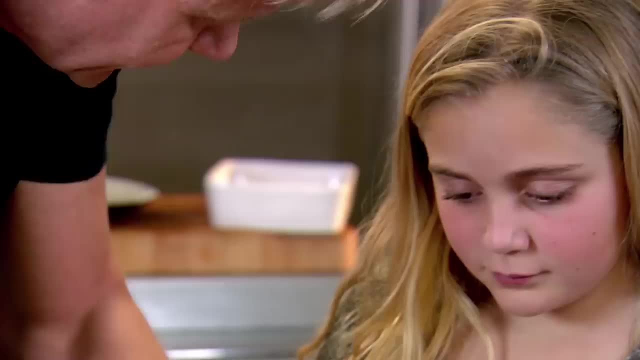 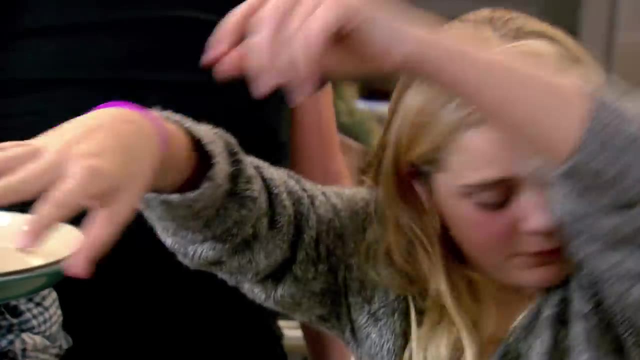 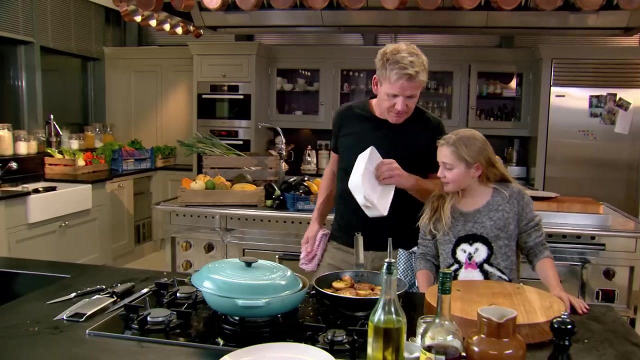 Now you've got all those wonderful flavours, You could almost be French Mmm. A little bit of that. Sprinkle that on there. Good girl, Nice, Merci beaucoup. Very yum, Nice. Now potatoes, Sounds like it's a chicken. 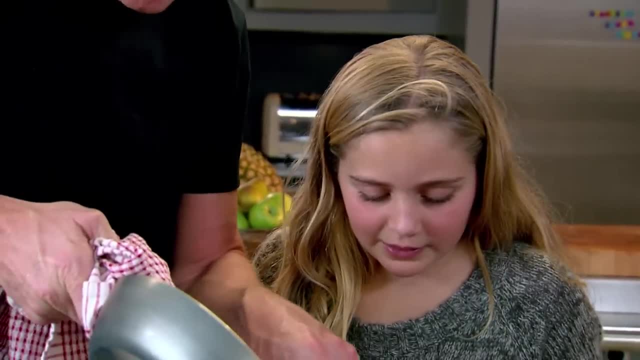 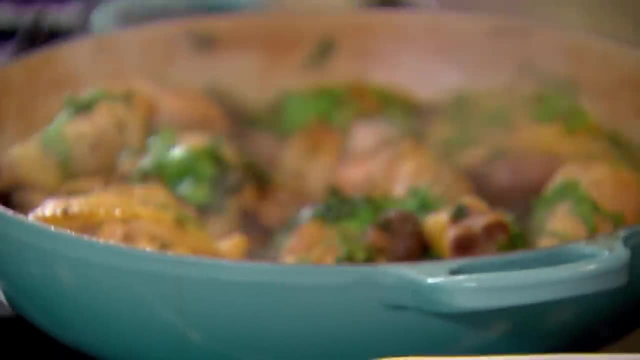 I can tell Jack's going to love this Is. he Looks delish, Doesn't it Smells delicious. Look at that, Mmm. You can smell that even before you took the lid off. That's good, my darling. 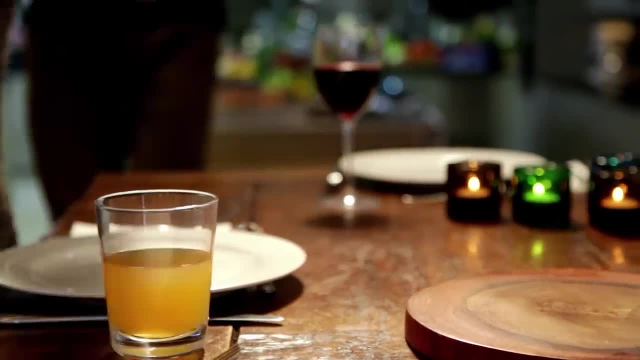 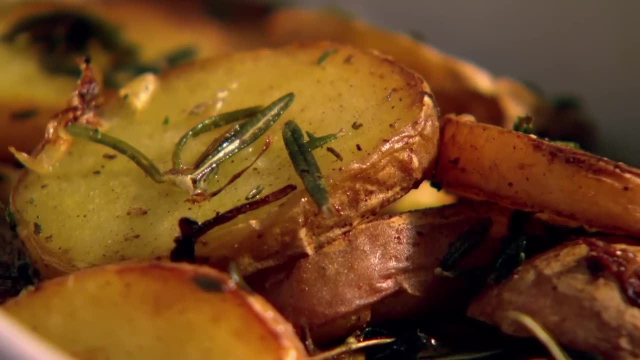 Good job, by the way. Thank you. I can't wait for the others to try it. I hope they'll love it. This is my ultimate French dinner: Chicken fricassee with sensational herby sautéed potatoes and lavender creme caramel. 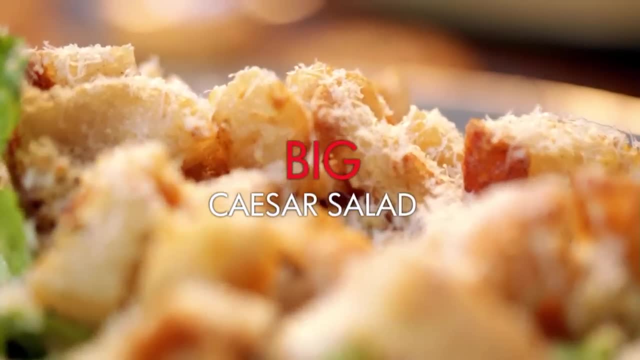 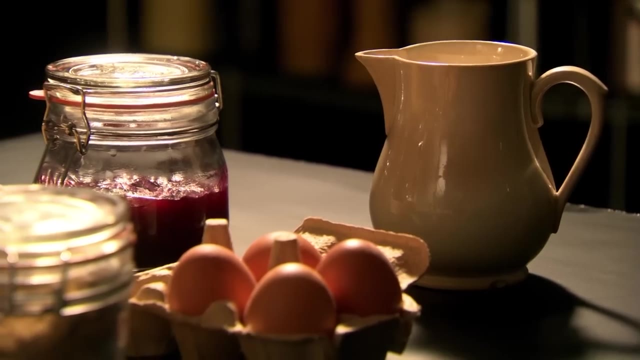 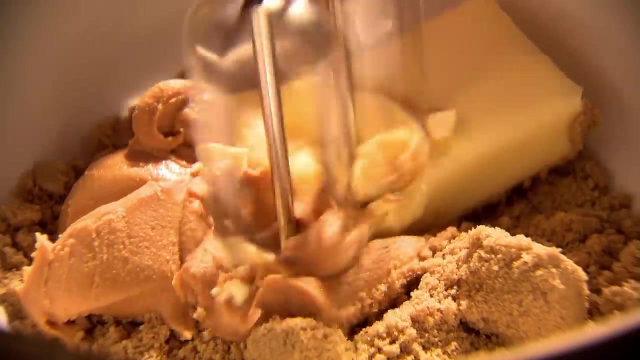 The main course will be a crispy big Caesar salad, But the first job are my peanut butter and jam cookies. Start with the cookie dough: Simply combine muscovado, sugar, peanut butter and butter until light and fluffy. Then add your egg, a splash of milk, vanilla seeds. 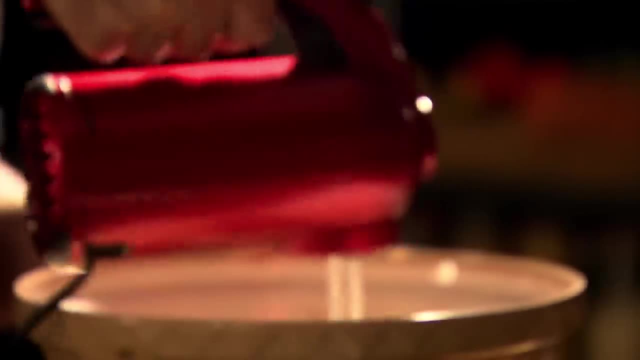 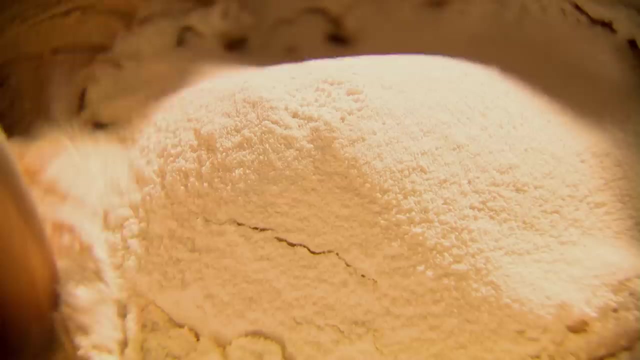 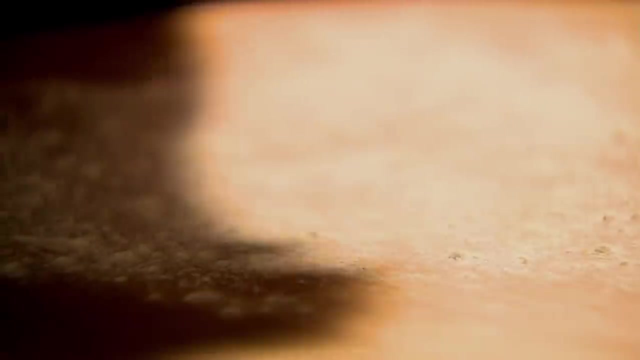 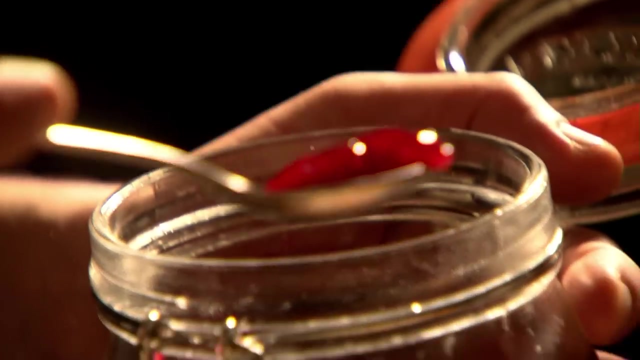 and beat again until smooth. Sift together salt, baking powder and flour, Then mix until thoroughly combined In floured hands. roll the cookie dough into golf ball sizes. Flatten and create an indent with your finger. Fill with half jam and half peanut butter. 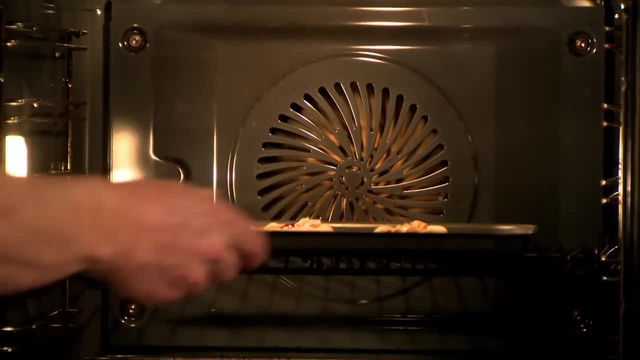 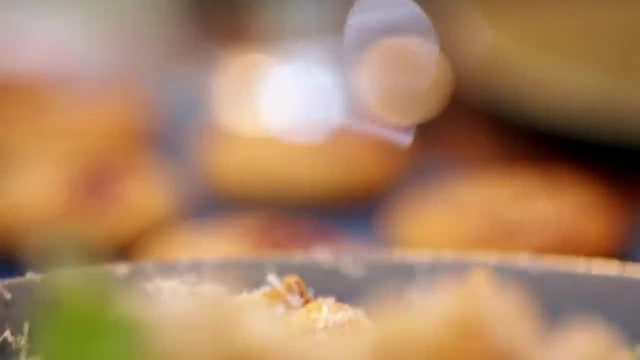 Place the cookies on a tray lined with baking paper and bake in a preheated oven for 10 to 12 minutes. Cool before serving Next job, main course, and my take on an iconic American salad first made almost a century ago. 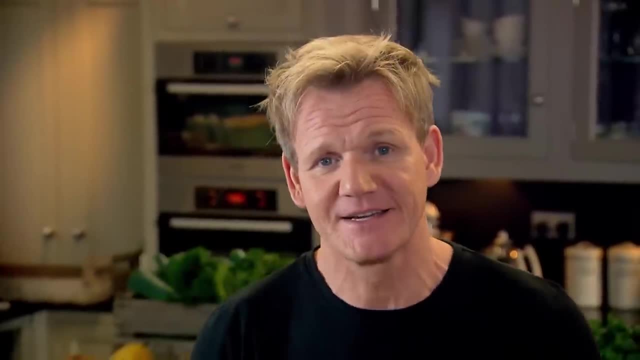 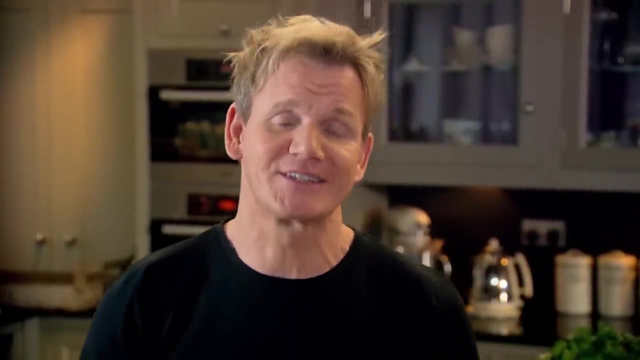 Caesar salad is definitely a classic, But the trick to keeping dishes like this modern and relevant is to tweak them but not lose what made them brilliant in the first place. Here's my version for the ultimate American lunch. My first twist is in the dressing. 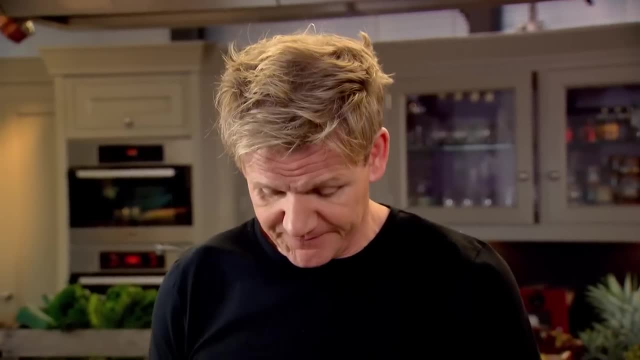 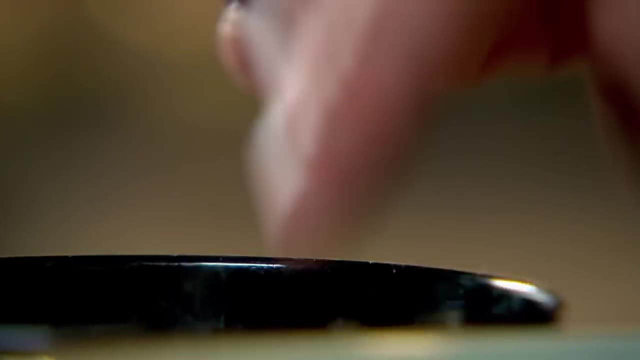 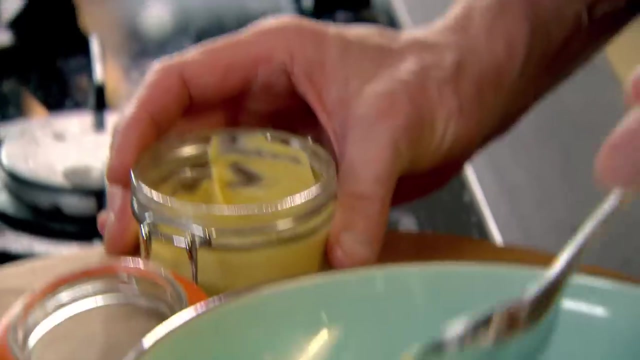 For me, the most important part of the Caesar salad is that dressing: Rich, creamy, slightly spicy. Begin by making a basic mayonnaise. Start off with the egg yolks In Just a little spoon of Dijon. 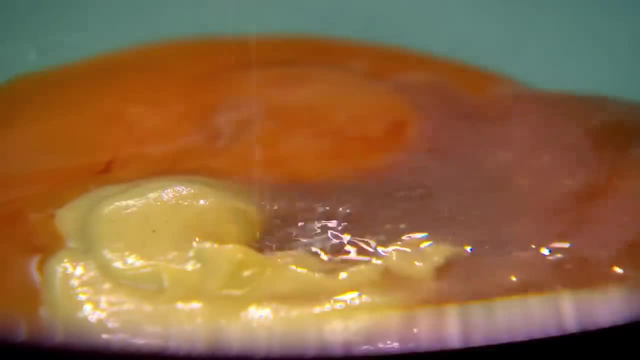 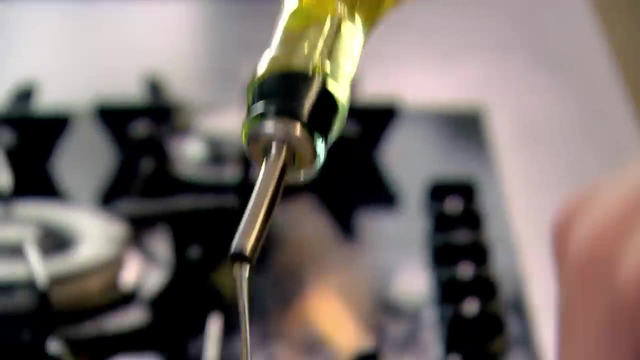 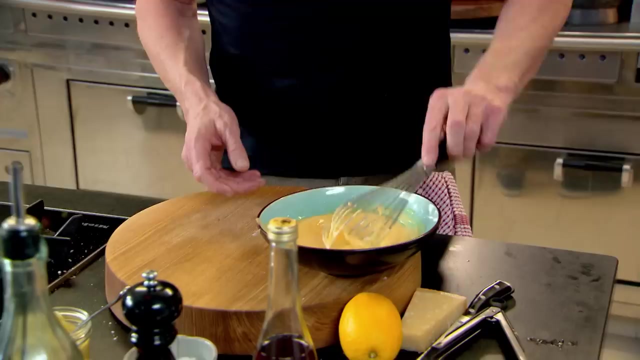 And then a little splash of red wine vinegar, Start whisking. Once you've got that nice slightly thickened texture, drizzle in your olive oil. It should fall through your whisk. It's like a nice thick double-cream texture. 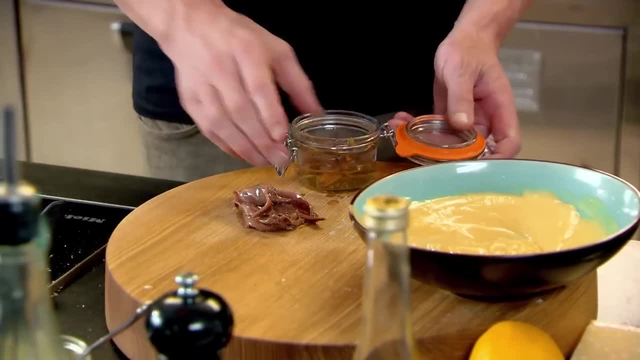 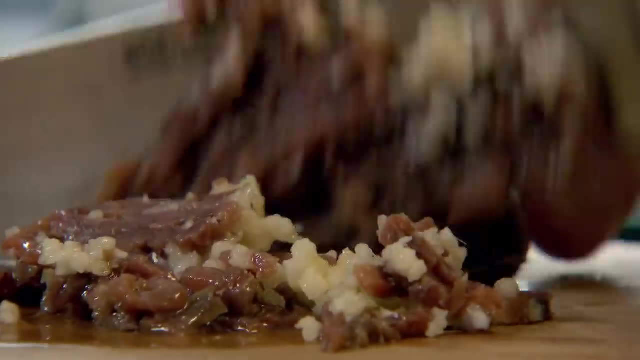 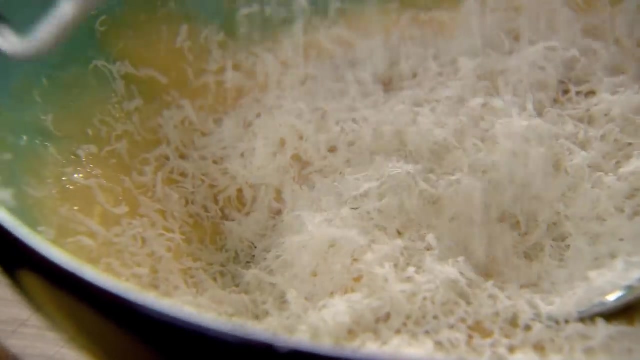 Beautiful. Now take the mayo to another level with anchovies and crushed garlic. Now chop up the anchovies and the garlic together. I sort of almost want that to be like a really nice puree, Then grated parmesan. 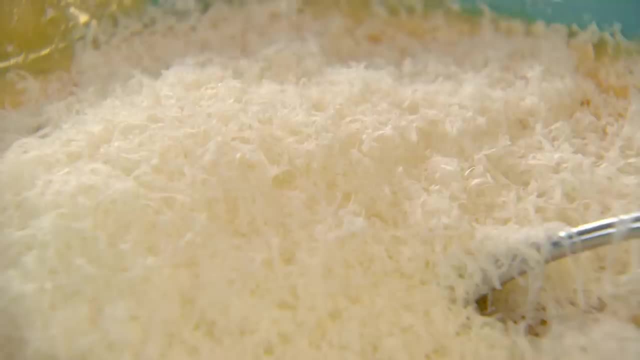 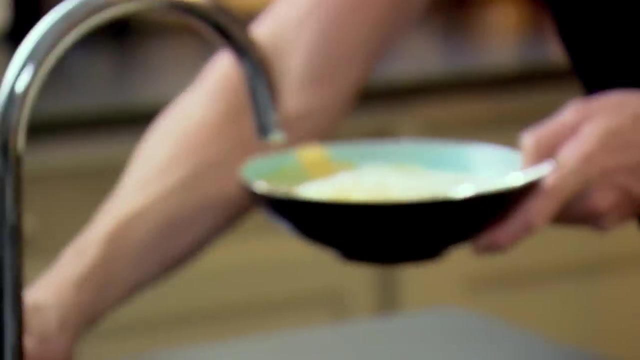 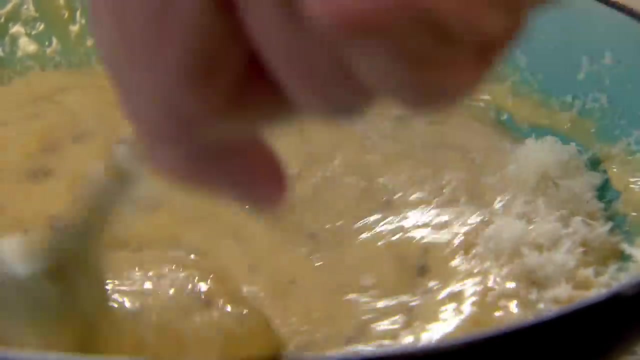 Lemon juice. That will make the dressing citrus-y, Lighter in colour, And then a little splash of water In. Now, all of a sudden, it transforms that mayonnaise into an amazing delicious. 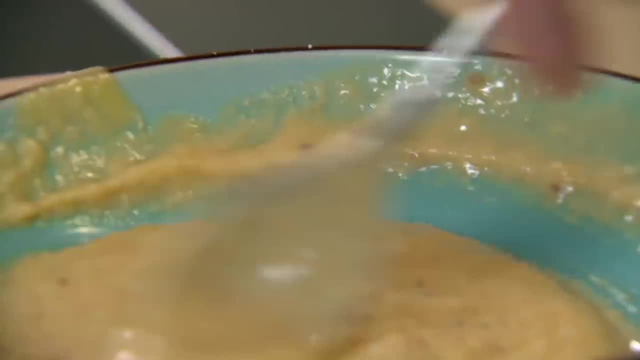 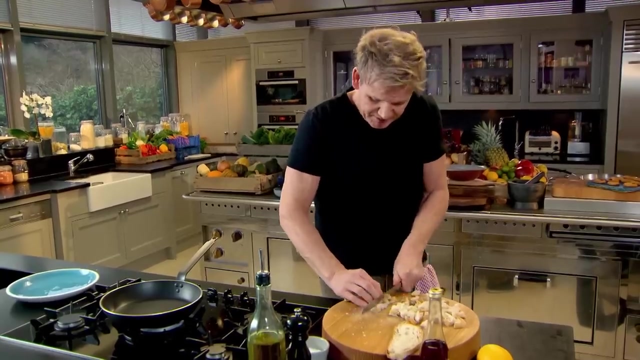 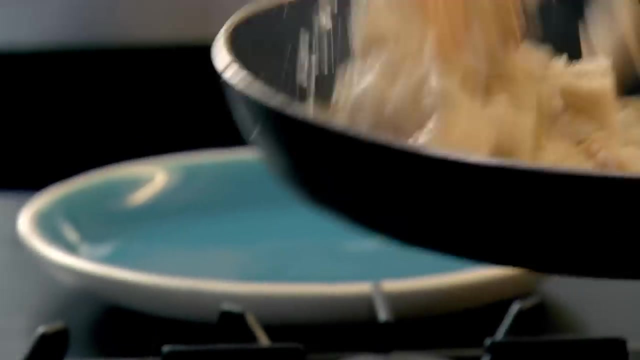 light dressing. Nice. Next job, the croutons. And I like using crusty bread for extra crunch And just dice up your bread Season with salt and pepper, then add to a hot pan with olive oil and fry. Give that a really nice toss. 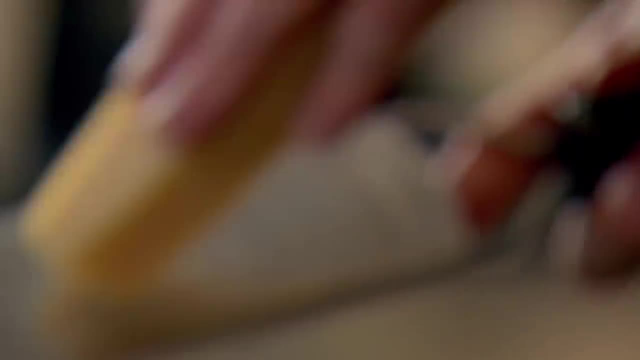 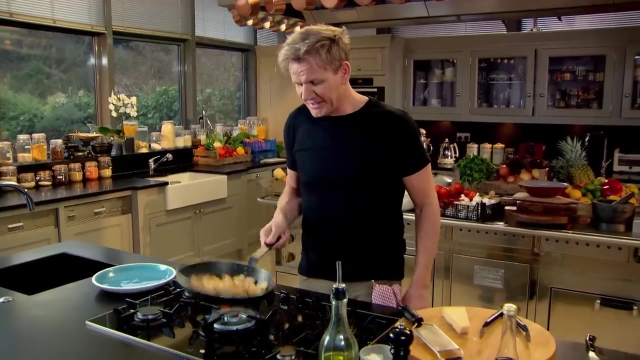 As the croutons start to turn golden, simply grate on a generous amount of parmesan cheese. Keep them rolling around. Stop them from sticking together. We've got that really nice, cheesy, delicious crouton. And now. 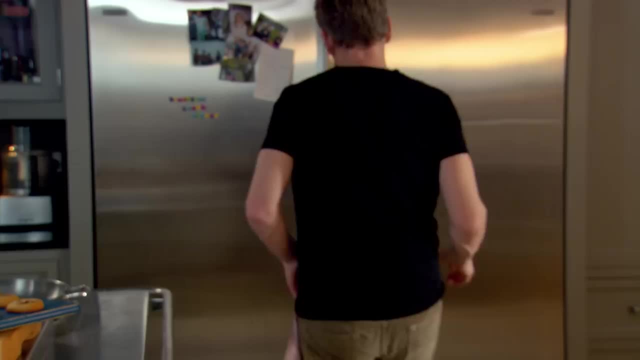 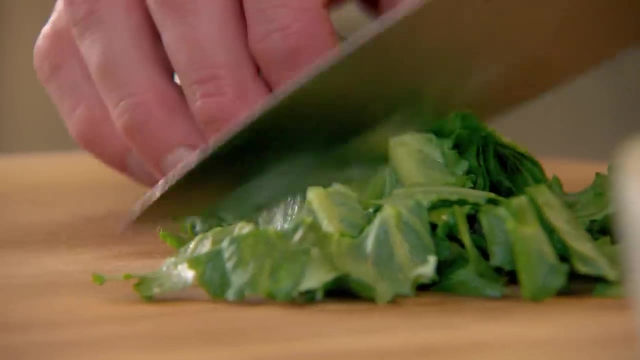 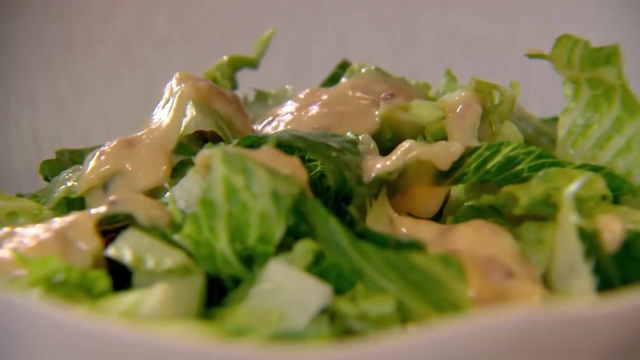 they're out Now for the fun job: Assembling the Caesar salad, Starting with the romaine lettuce- And don't slice the lettuce too thinly. A squeeze of lemon On with half of that gut sauce, Then add in the sea anchovy mayo dressing. 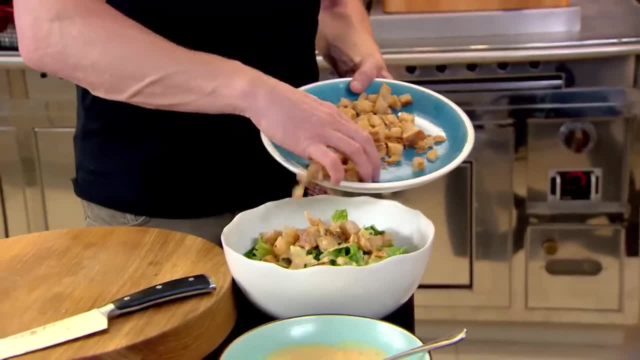 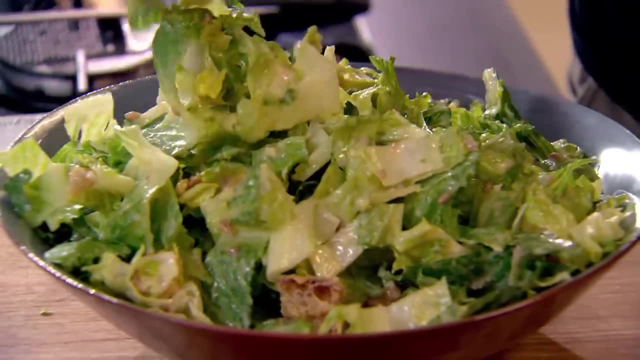 Saving some to coat your chicken later. Then sprinkle half your croutons. Give that a really nice mix Salad in. It's all beautifully dressed. Add the remaining croutons and finish with a good grating of parmesan cheese. 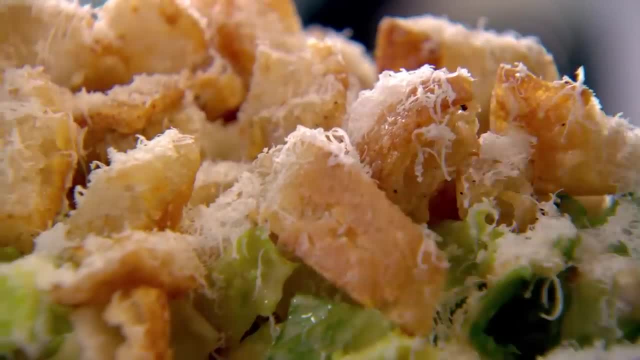 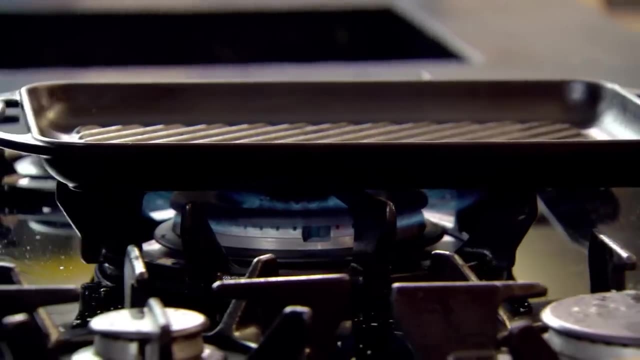 That, for me, is a perfect Caesar salad. However, I'm going to take it to another level and grill a stunning chicken breast. Start by preheating your griddle pan, then butterfly your chicken breast. Simply slice from the thin end towards the thick bit of the breast. 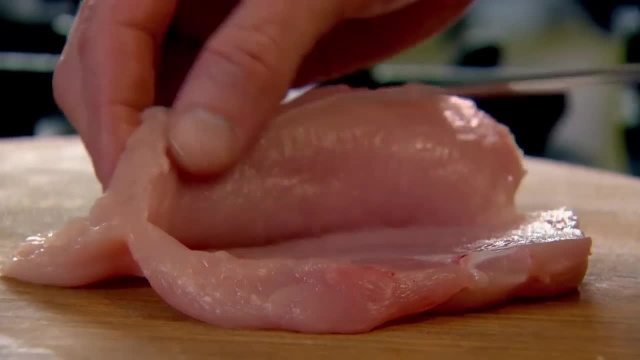 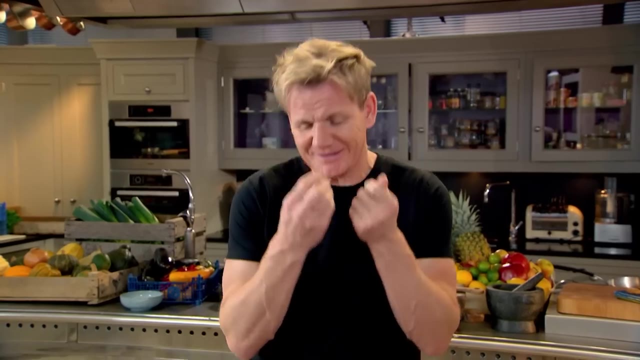 Let the knife do the work and literally just open up. Now that's how we butterfly a chicken breast, So therefore it will cook twice as quick and just nice and moist in the centre. Season the chicken on both sides with salt and ground pepper. 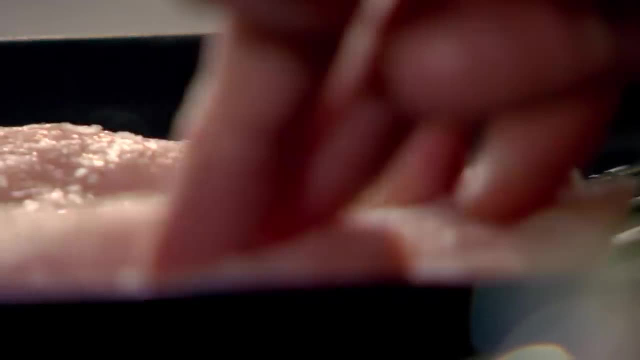 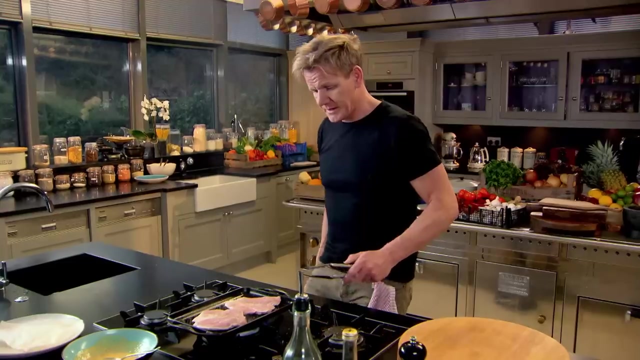 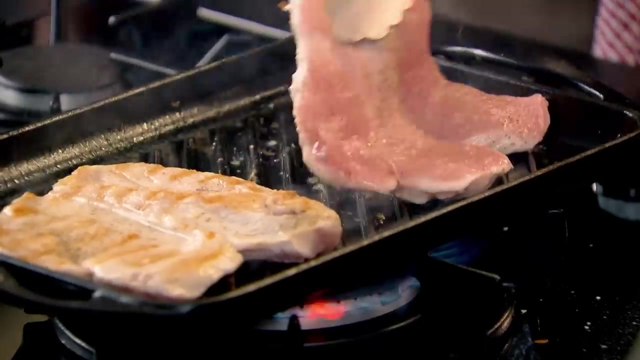 Lay your chicken breast onto the grill. CHICKEN BREASTS GRILL. Never oil the grill until you're absolutely ready to cook your chicken. Now turn them over There, Beautiful. Cook for three to four minutes on each side until the chicken's got those lovely stripes from the griddle. 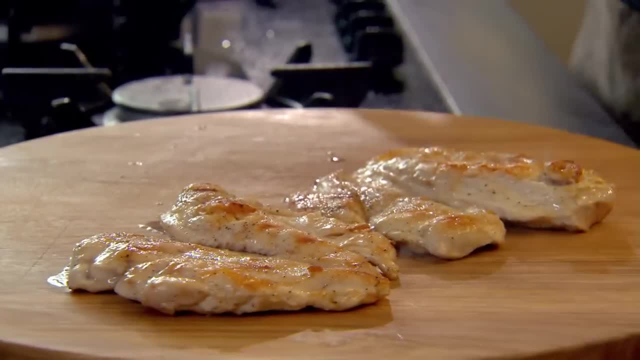 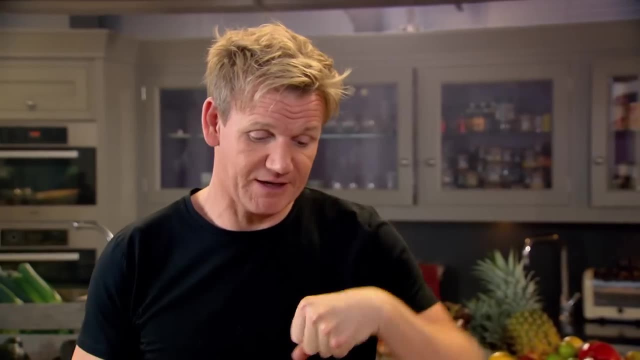 which adds a gorgeous smoky flavour. Whilst they rest spoon over some of the remaining anchovy dressing, The chicken cools down The flavour. the seasoning of the anchovy, the garlic and the parmesan seeps into that chicken. 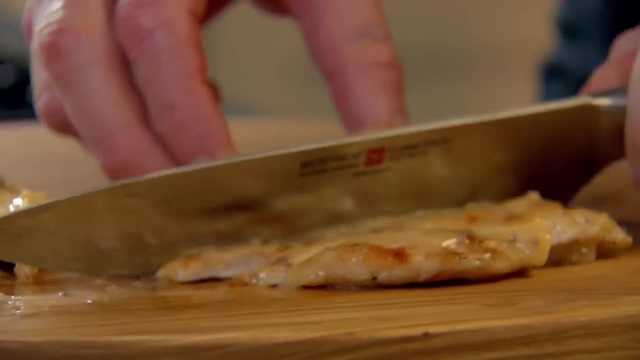 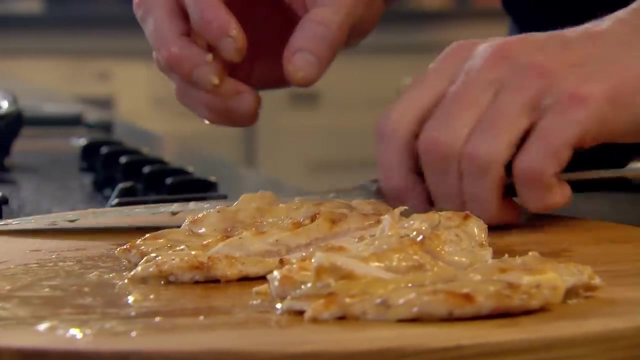 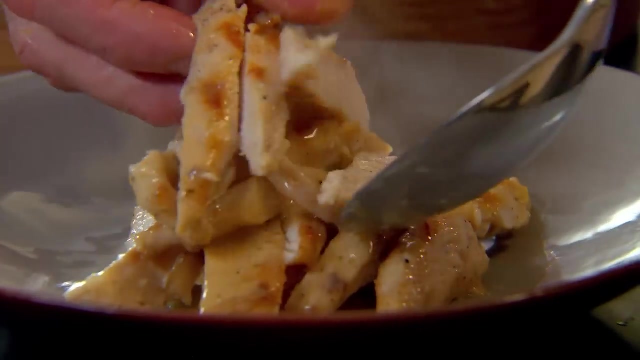 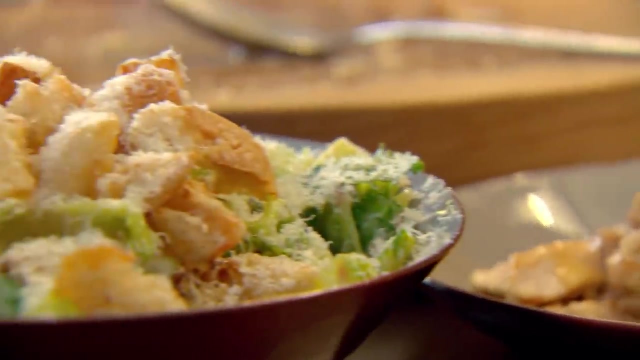 Slice the chicken into strips. Mmm, Wow. I serve the chicken warm in a separate bowl so it doesn't wilt. the salad Spoon the dressing. Finish that with a little touch of dressing. An American classic and, I think, one of the most popular salads anywhere in the world. 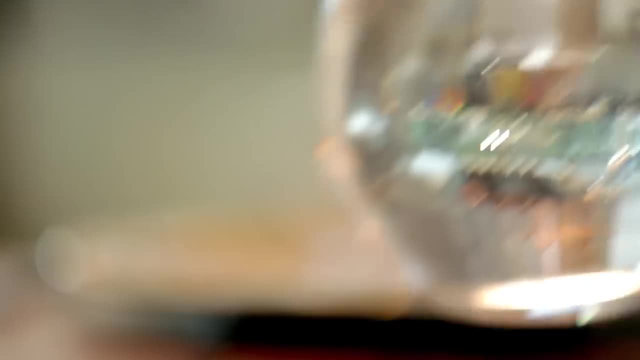 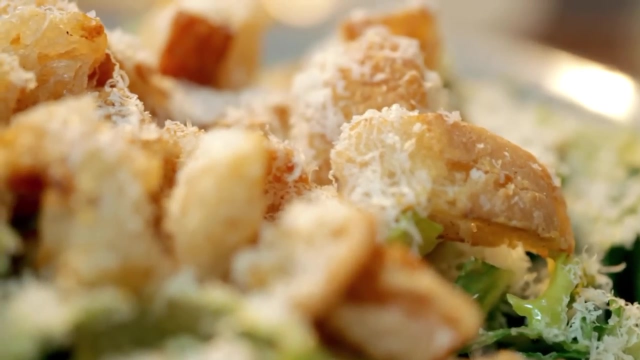 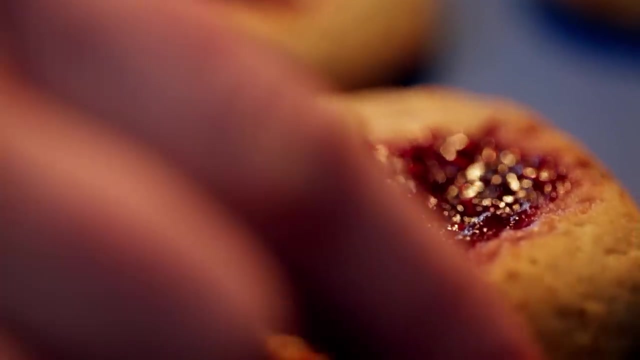 But it's still one of the most delicious. When it comes to lunch, this really is an American dream: A delicious Caesar salad and succulent golden griddled chicken with peanut butter and jam cookies for dessert- Your favourite chicken thighs. First of all, we'll turn on the grill. 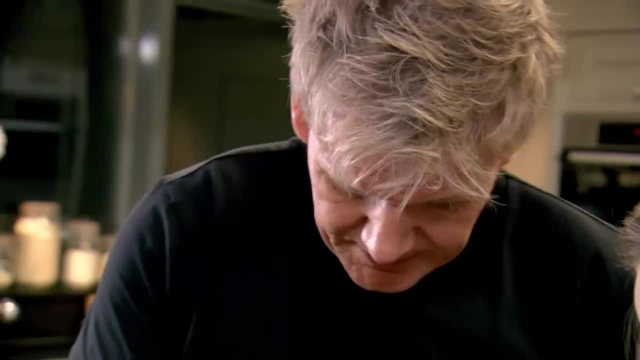 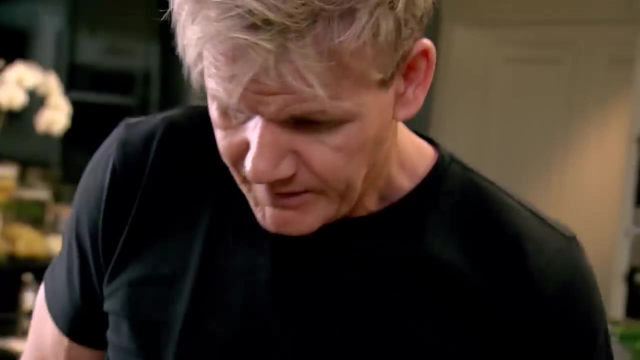 The reason why we're using the thighs, ie the brown meat, is so it doesn't go dry. Season them nice Salt pepper Olive oil, Then turn them over. please Go on, get your hands in there. 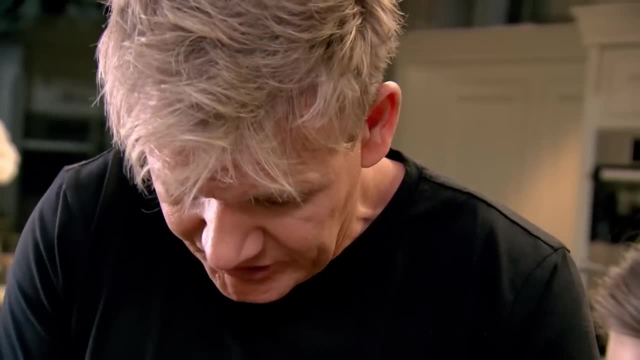 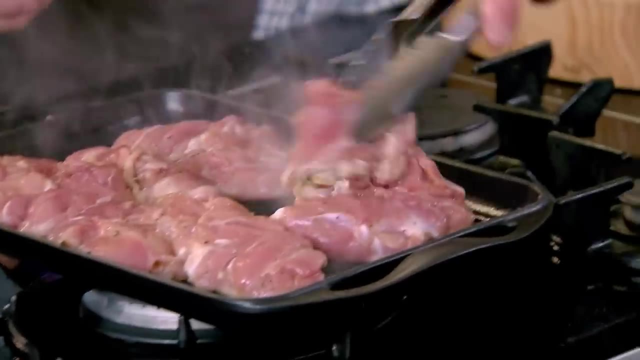 Good, Don't worry about your nail lunge, So there's no bones in there. so the chicken will cook really quickly. Why do you do it skin side down? Skin side down first. That'll stop the chicken from going dry and it'll get it really nice and crispy. 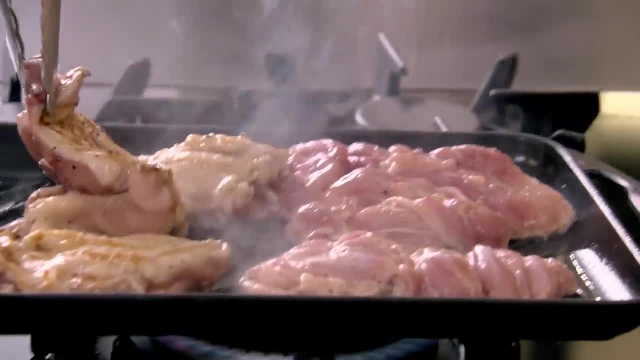 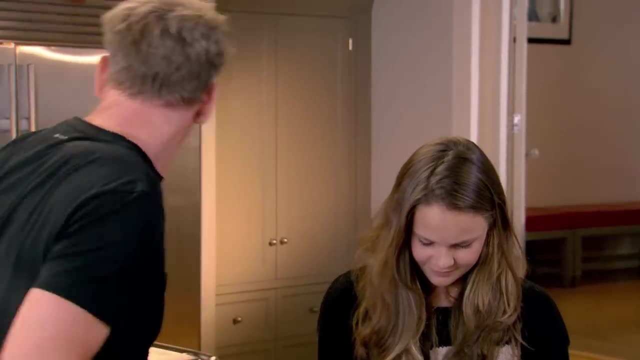 Turn that over. Good, See the way it's marked the skin now. Yeah, Got all that really nice flavour in there as well, And we'll turn them every two or three minutes. How much do you love chicken? Lots, Lots. 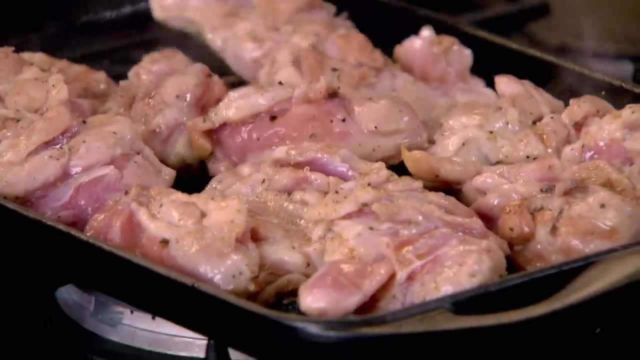 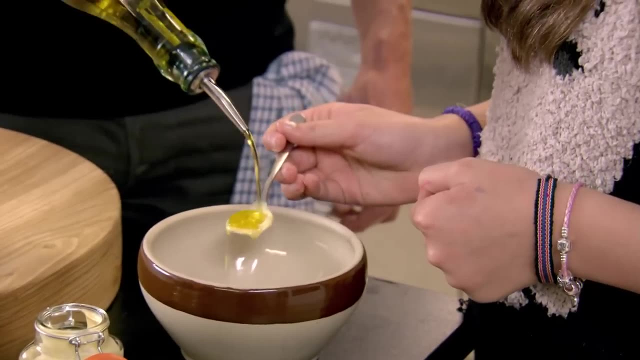 Lots. We'll serve that with some really nice chickpeas. First of all, we'll make a little dressing. OK, One nice teaspoon of mustard in, please, A little bit of olive oil, A touch of salt and pepper. Give that a really good mix. 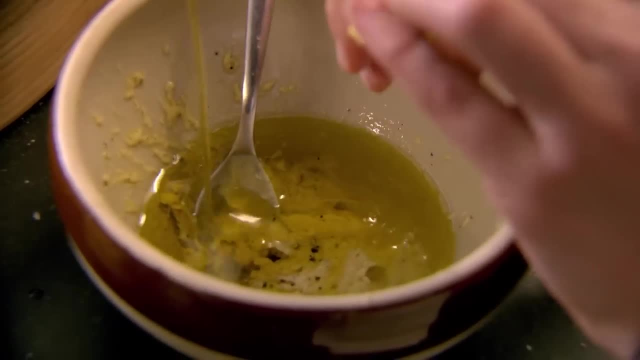 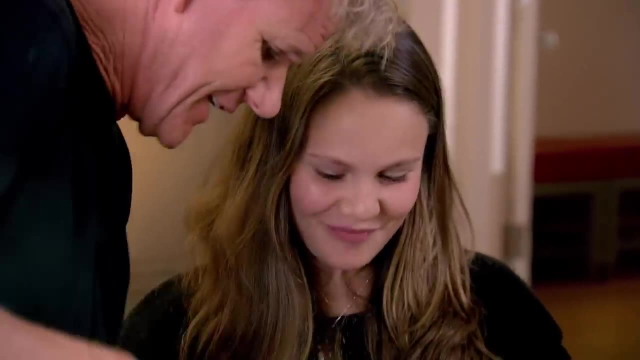 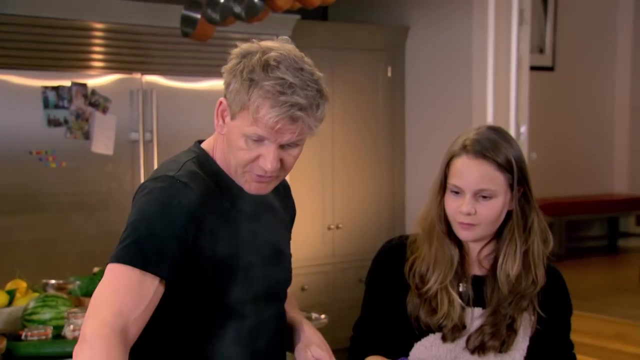 And then just squeeze lots of lemon juice in there. A little taste, That's nice. Mmm, That is delicious. Now look at that chicken. now Follow that. Beautiful, Nice and crispy as well. Turn the gas down now and leave that chicken to griddle. 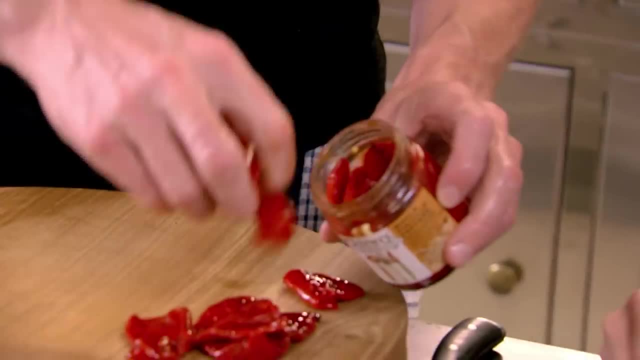 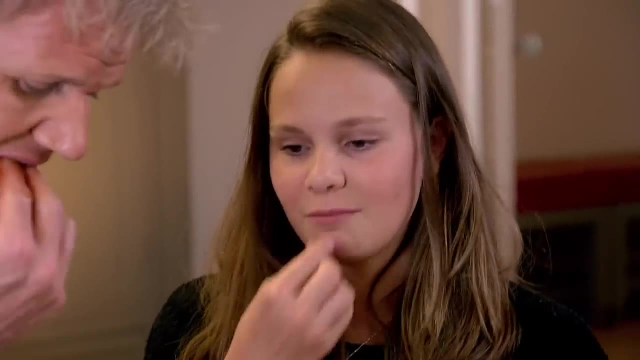 Right, let's get the chickpeas done, shall we? Yep? So we've got poquillo peppers. So these are roasted, smoked Spanish peppers. Have a little taste, Mmm, I would like you to chop up the quesadillas. 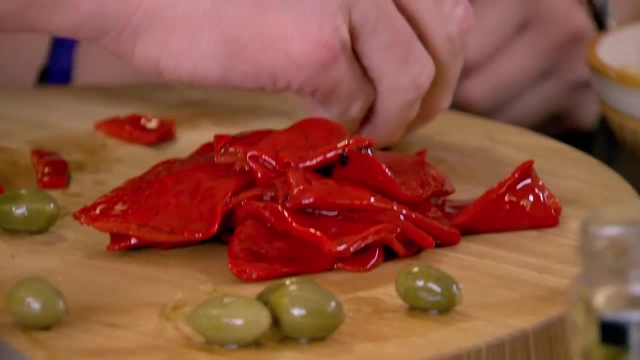 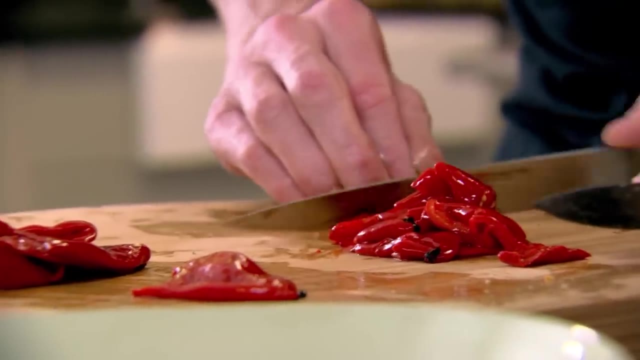 You take off the top, I'm going to slice them in half like that. Watch your fingers, I will. OK, So these are small poquillo peppers. Yeah, A bit sweeter. There you go. Watch your fingers, please. 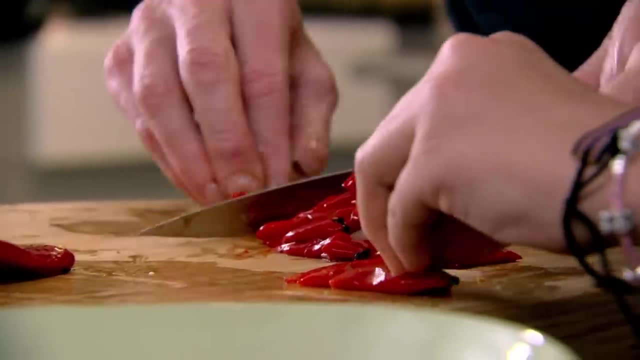 Watch your fingers, please Tuck them in. Three-finger rule. Come on, Holly, You know the three-finger rule. I've been telling you that since six months old. Good girl, You're fast, aren't you? 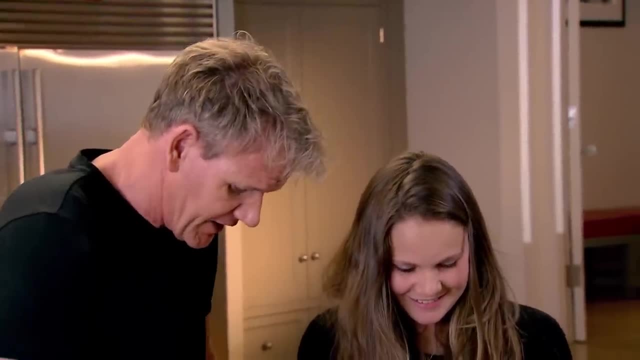 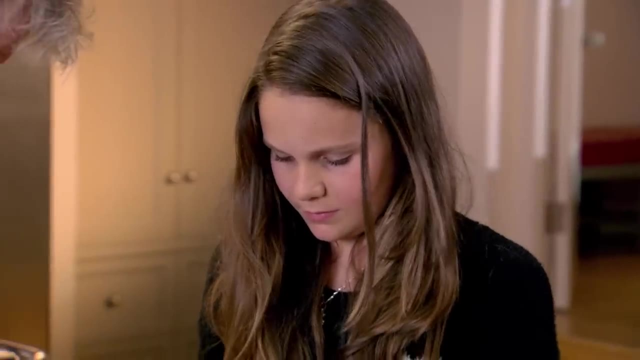 Yeah, In fact you're faster than Jack. Don't tell him, It'll get him upset. Shall I put the peppers in? Yes, please, Thank you Good, And then give it a little mix with your fingers, Please. 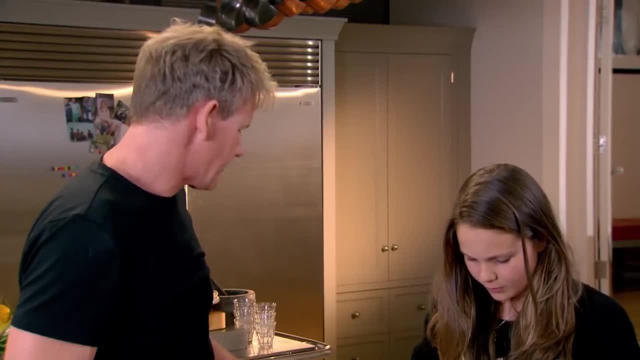 Lovely Rump holes Out. Come on Out, out, out. OK, Get out. Every time there's food, he's always there. He smells it from a mile away. The chicken's grilling skin side down. 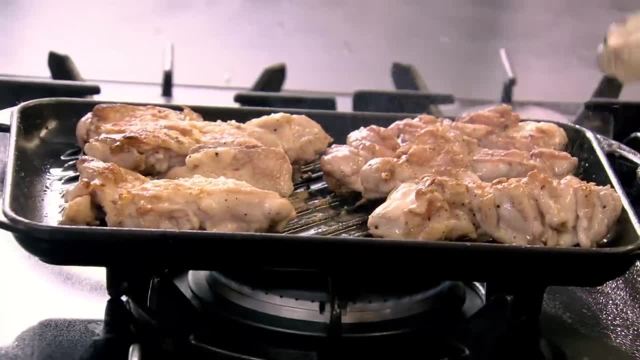 Why is it on skin side down? Because it keeps it moist, Keeps it really nice and moist. That's right Now. we'll start the watermelon salad. Watermelon feta, cucumber Pan- nice and hot, Get the pecans. 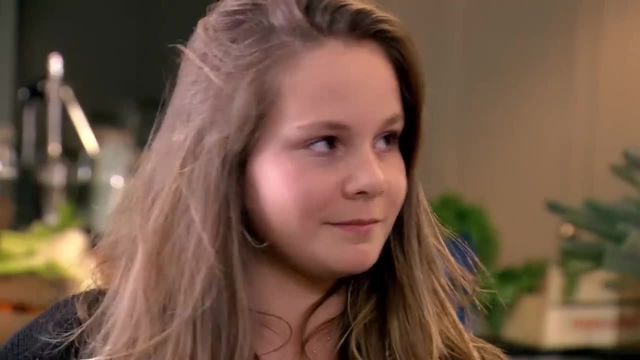 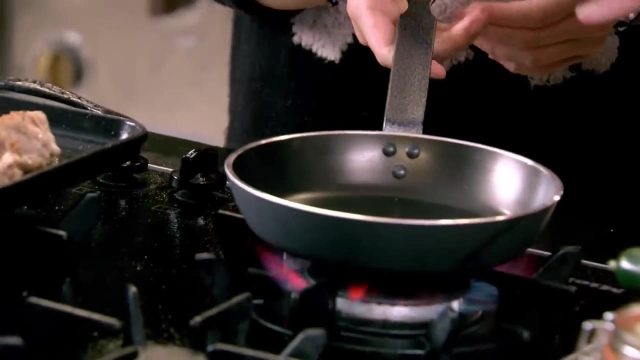 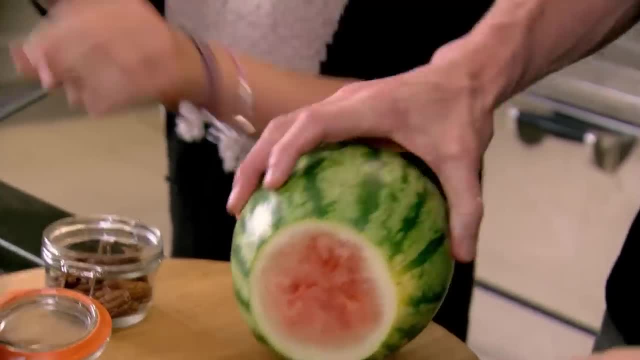 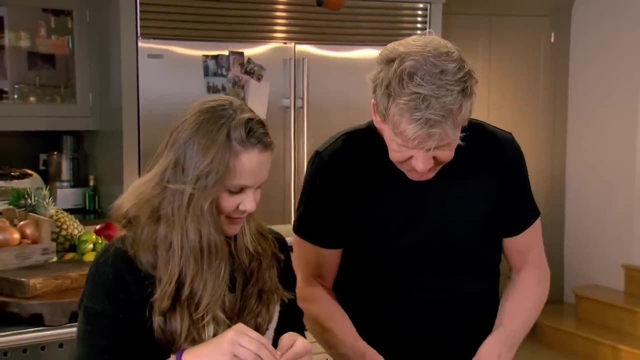 OK And just sort of break them up. I'm going to start slicing the watermelon. Do you keep the seeds in? Yeah, The seeds are fine. So you just make these little boats and go around like that. Now, with the toasted pecans, give them a little seasoning, would you please? 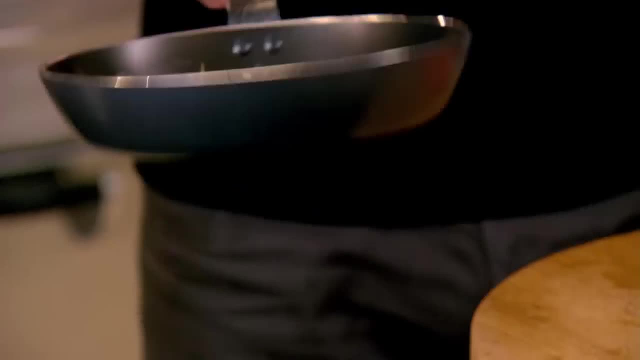 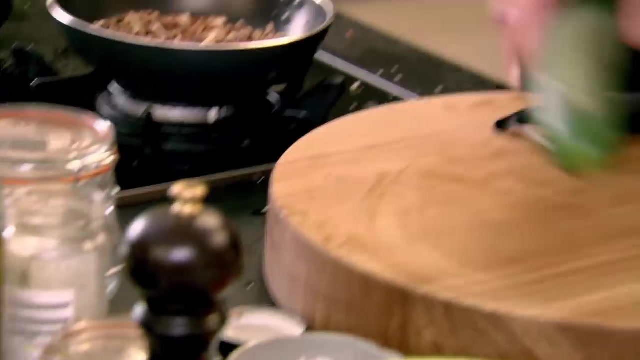 With pepper too. No, just a touch of salt, Thank you. Roll them around And just start to see them smoking. See, Now turn the gas off, please. We're just going to take half the cucumber and give that a little peel from it, please. 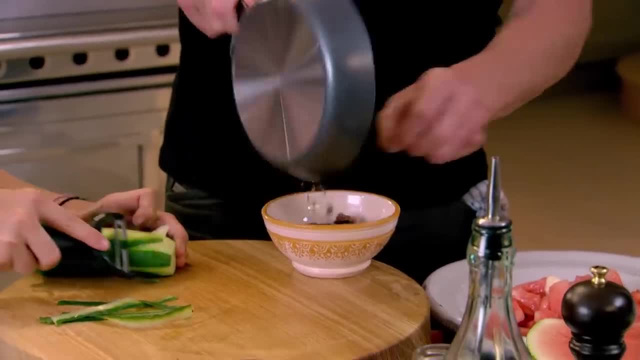 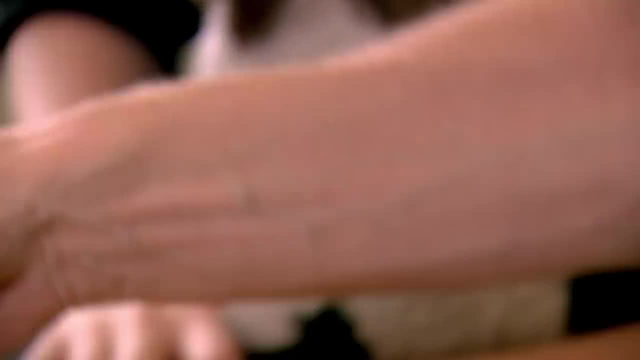 That's nicely dry roasted. OK, Take them off. So from there. I want you then to slice around the seeds, And that's the watery part. OK, We'll keep that out. Wash your fingers, please, Nice. Am I still faster than Jack? 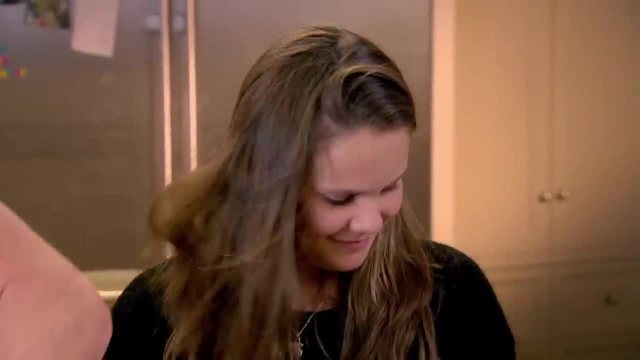 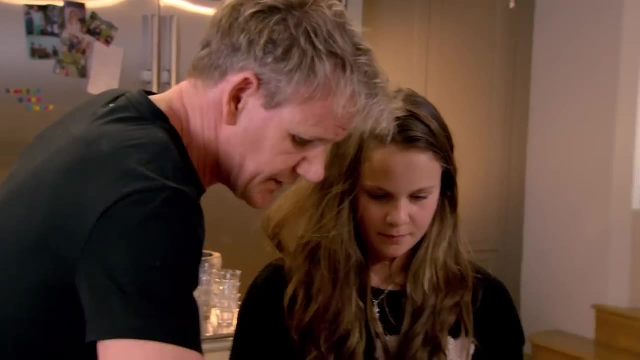 You are still very fast, A lot faster than Jack. Now cucumber on top of the melon. We'll mix it up in a minute. I want to give that a nice little light seasoning. A touch of salt and a little touch of pepper, please. 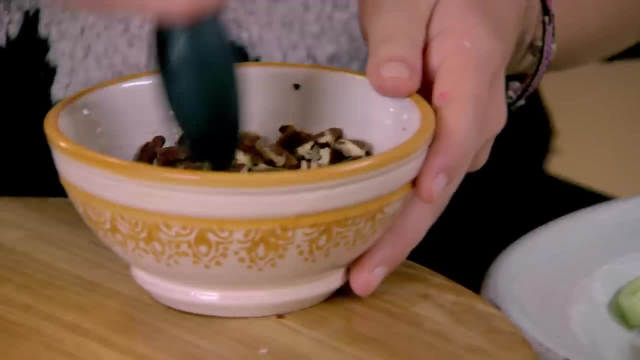 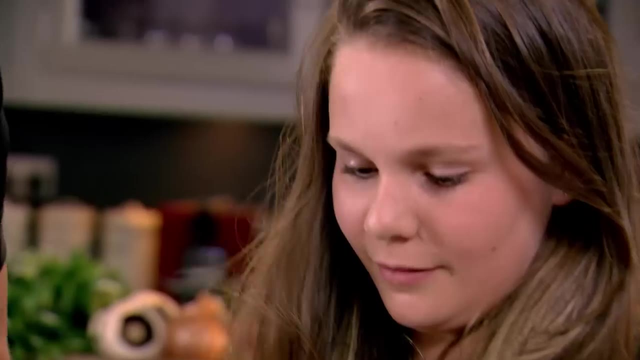 Crush those little bits Pecans in there for me. Nice Next Greek feta cheese. This is kind of easy, Isn't it? Jack? That fat lump snoring. You've got to get him out of here. Hurry up, mate. 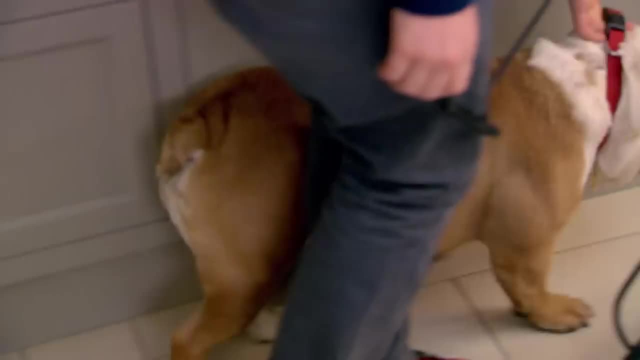 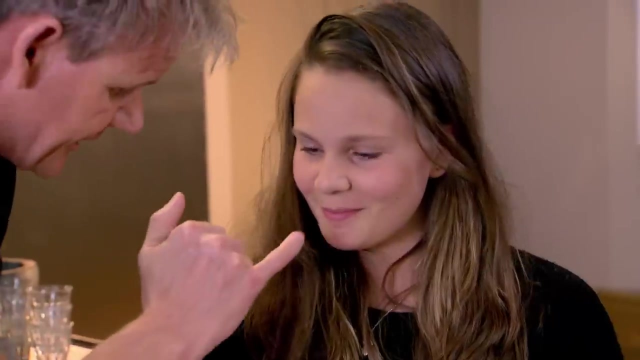 Take him out. Fat lazy lump snoring his head off, Come on Out. So we've got that nice juicy melon, the cucumber and now the cheese. We need something to bring it to life. Have a taste. 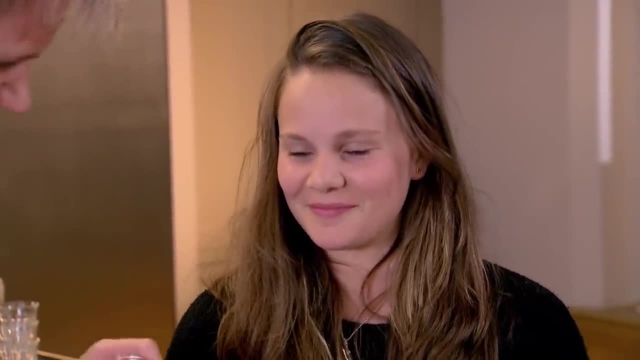 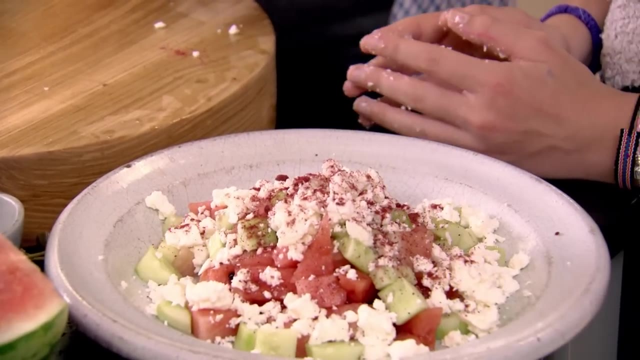 That's sumac. OK, OK, That is very citrusy. We're just going to season that lightly. Now what I want you to do is sprinkle the pecans in there. Mmm, What's that? Basil, Mint, Mint. 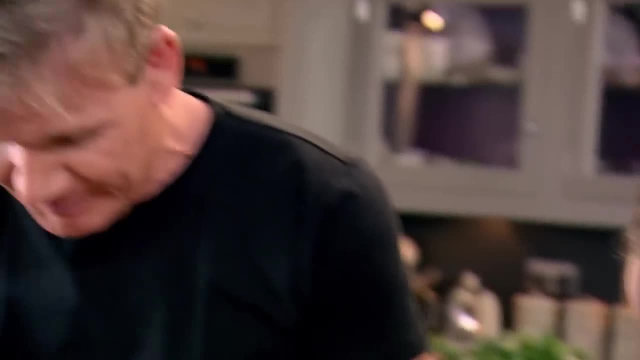 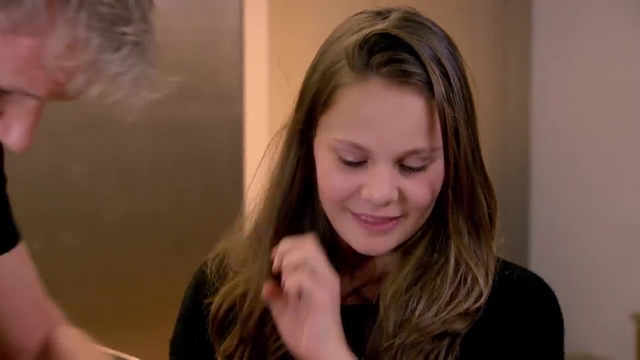 Sorry, Minty. Sorry, You're getting confused with Basil, your boyfriend. No, Daddy. OK, Good, Keep it that way for another ten years. Fresh mint over And then a little drizzle of olive oil. OK, That's it. 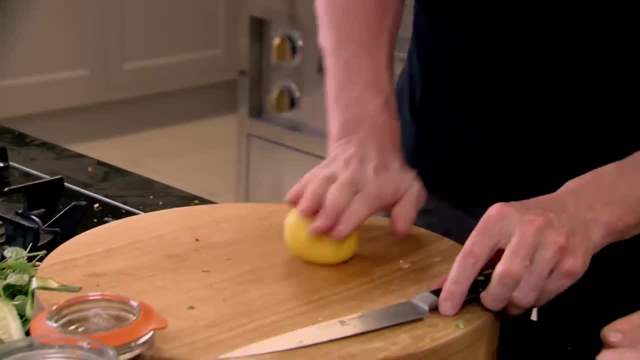 Yeah, I know You're dying to get in there, aren't you? Mm-hmm, And just some fresh lemon juice. Why do you roll it? It starts to release all the juice. You can now feel it, So it's less firm, a little bit more squashy. 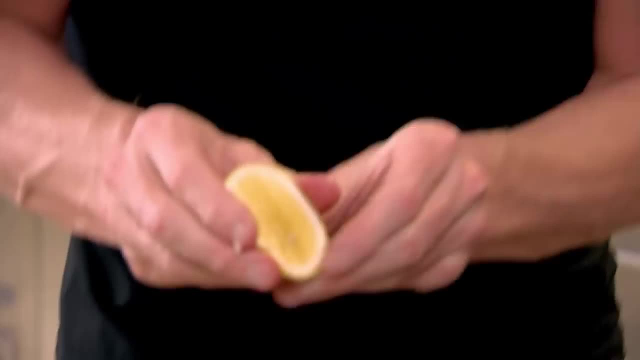 Now it's all that lemon juice coming out. Now, what I'm going to do is just have a little taste, Mmm, Mmm. What do you taste? Everything, yummy, It's fresh, isn't it, Mmm? So that's the salad done. 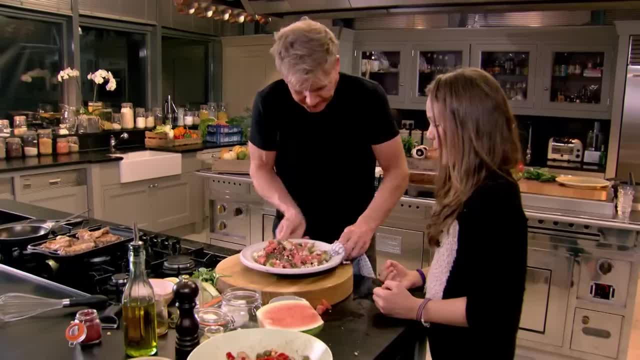 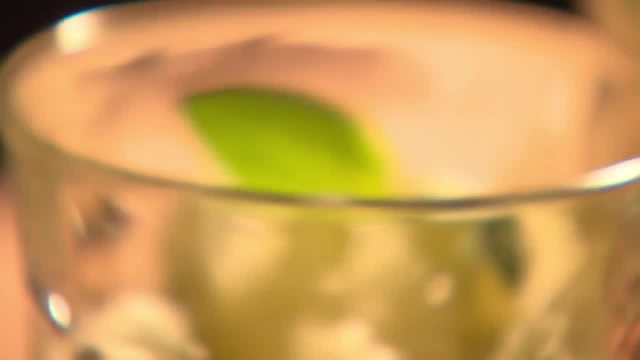 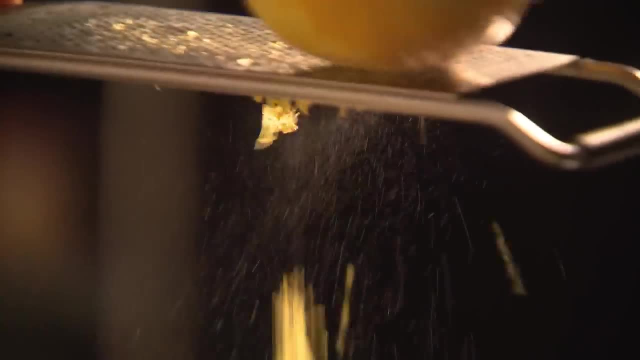 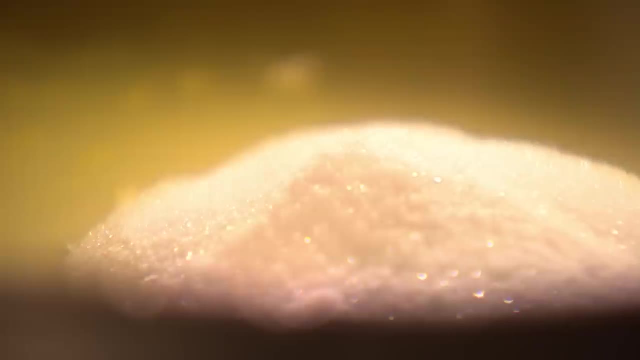 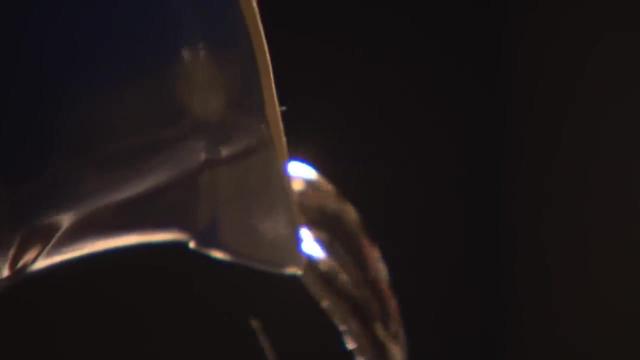 Start by putting the juice of seven lemons and the zest of one into a small pan with a sprinkling of caster sugar. Stir over a medium heat until the sugar dissolves. Dilute your granita mix with a little water. Pour into a freezer-proof container. 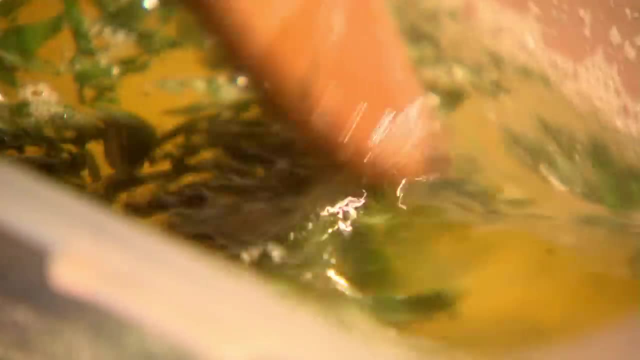 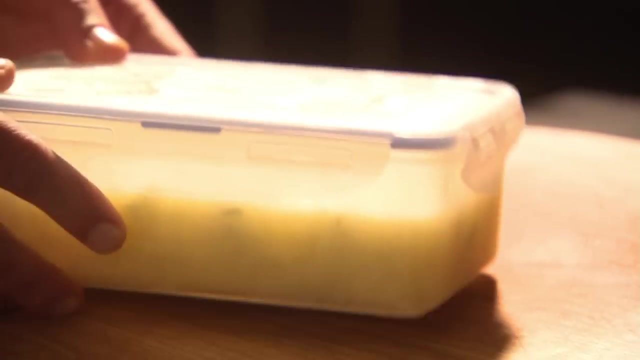 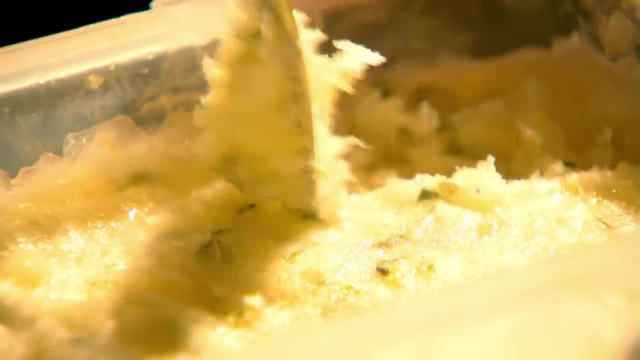 Stir in a good handful of chopped fresh basil and place covered in the freezer for three hours. When the granita is frozen around the edges, lightly break up the mixture with a fork, Return to the freezer and repeat twice until the granita is frozen with a granular texture. 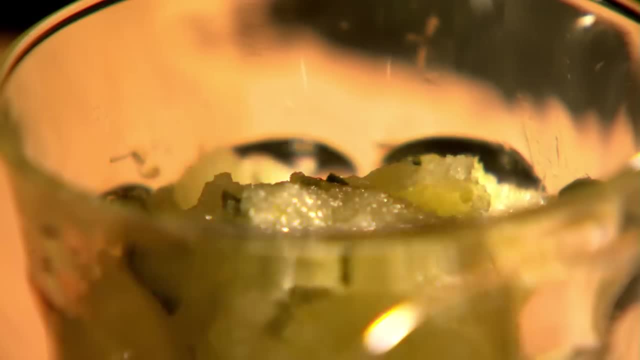 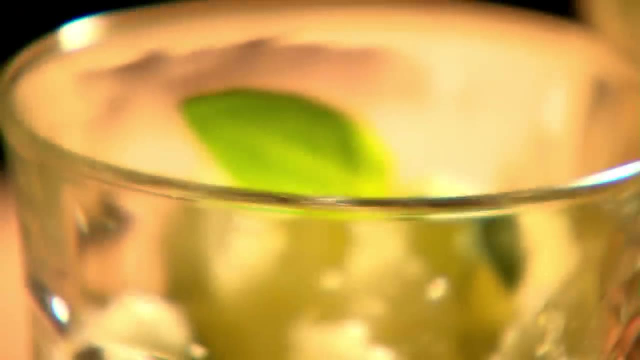 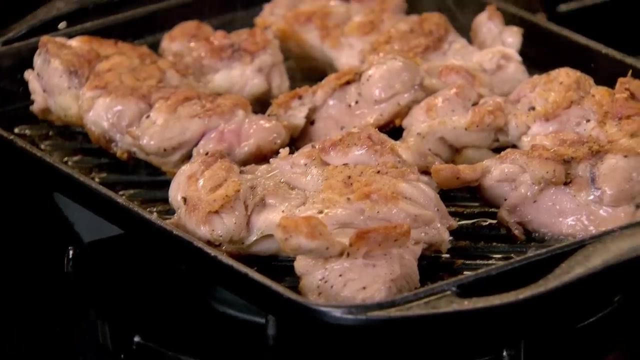 Spoon into chilled serving glasses, Garnish each with a sprig of basil. OK, Amazingly light and refreshing lemon and basil granita. With our granita and feta salad done and the griddled chicken beautifully charred, we can put the final touches to our main course.